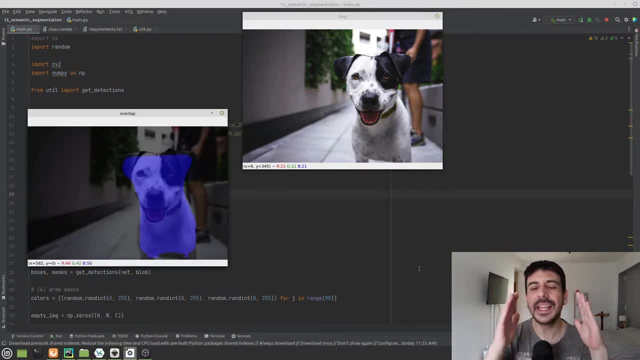 image, and the output is going to be a mask with the exact location of all of our objects in this image. For example, in this case, we are taking an image of a dog. this is an image containing only one dog and the output is the exact location of where the dog is located. So this is the project. 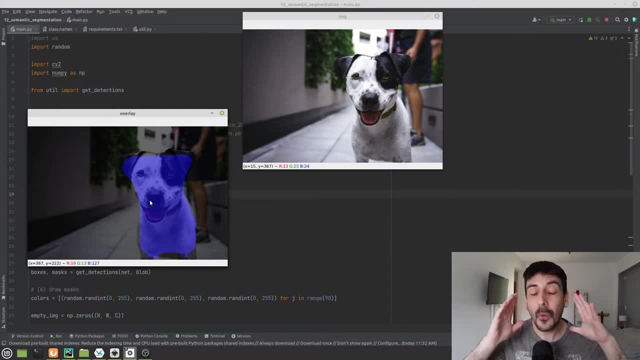 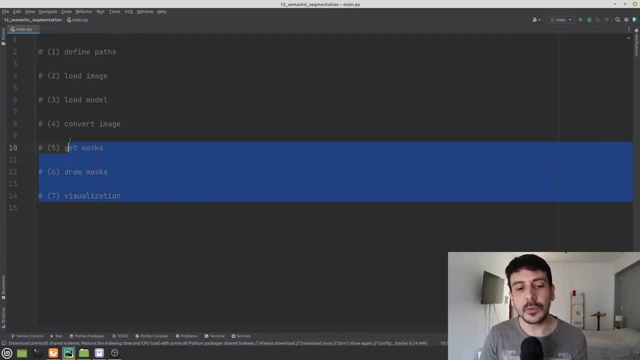 in which we are going to be working today, and we are going to work 100% with Python and OpenCV. So let's get started with today's tutorial. This is the process in which we are going to be working today. You can see, this is only going to be a seven steps process, so this is going to be very fast. 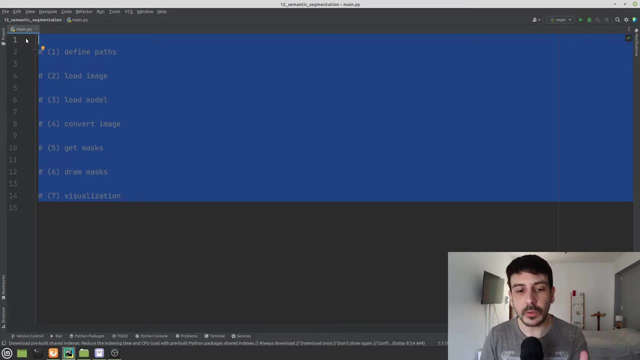 very easy. it's going to be very, very, very straightforward, and I'm going to walk you through each one of these steps. Let's get started. This video is going to be very, very similar to one of my previous videos, where I show you how to implement an object detector using Yoruby3, Python and OpenCV. 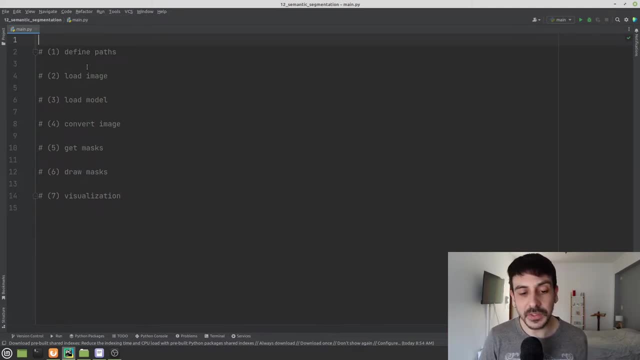 So this is going to be a quite similar process. this is going to be a very similar tutorial, and if you haven't watched that video, I strongly recommend you to watch it, because it's a very good video. it's a very good tutorial, so I recommend you to watch it before. 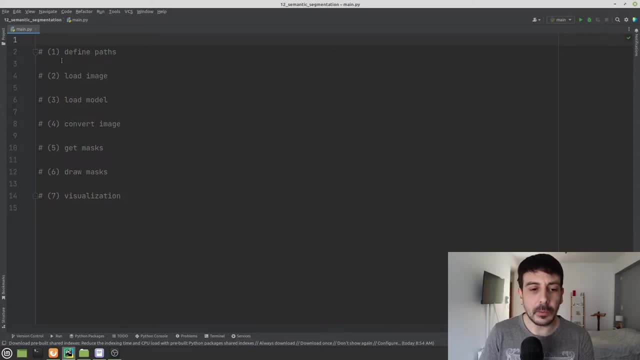 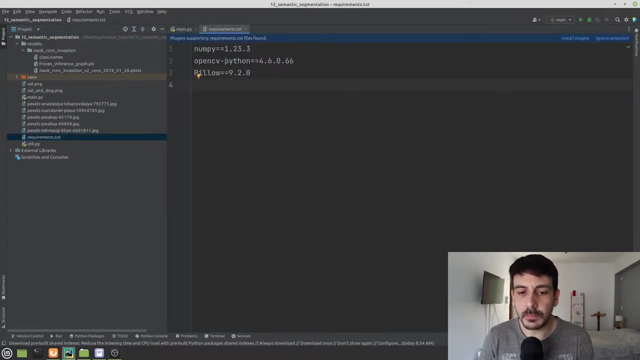 starting this tutorial. Now let me show you a couple of things Before starting, and I'm going to show you the requirements which we are going to be using today. We're going to be using numpy, OpenCV and PILO- I'm not sure how to pronounce this library. 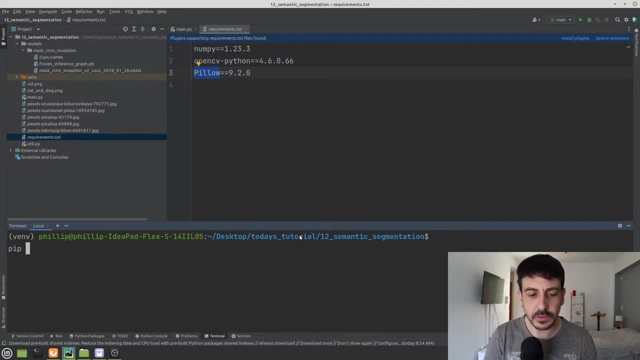 and the way we are going to install these dependencies is going to be, as always, going to the terminal and type in something like pp install minus r requirements. In my case, I have already installed these requirements, so nothing is going to happen on my computer, but please remember to install these libraries before. 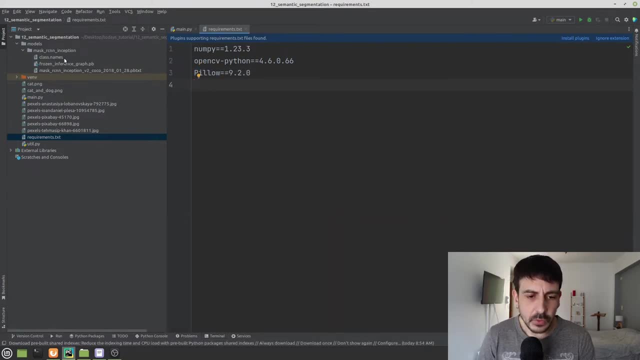 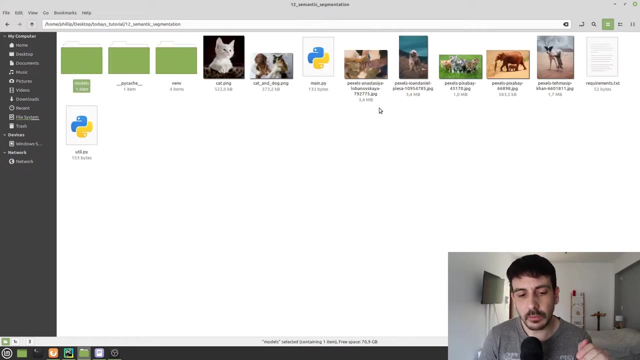 starting the tutorial Now let me show you the model which we are going to use, and maybe it's best if I go to my file system. This is the. this is a repository I created for this tutorial, for this project, and this is the model which we are going to be using today. 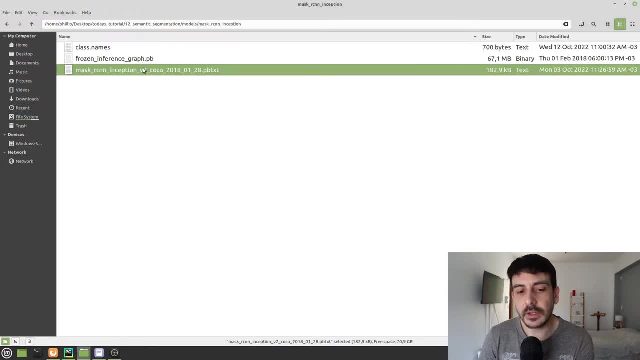 It's called maskrcnn-inception. Inside this directory I have three files. one of them is the file which contains all the weights of our model. the other file is the one defining the model itself, the architecture of our model. and then we have another file which 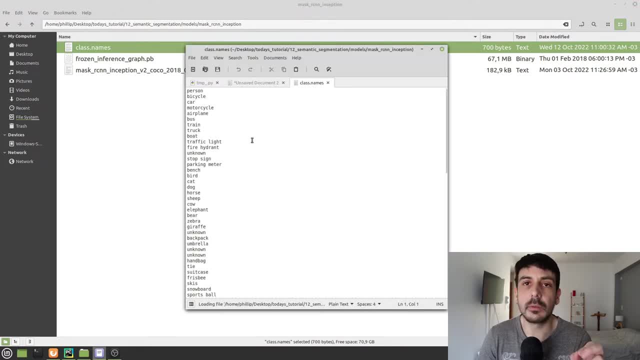 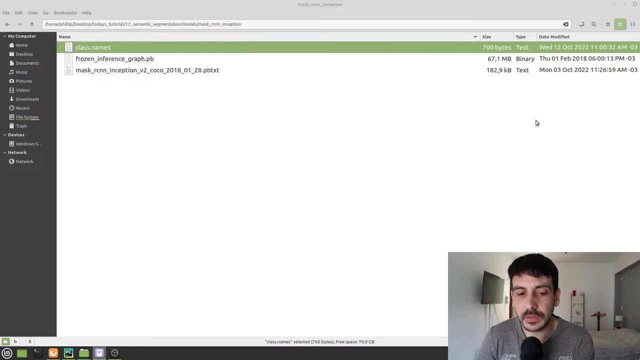 is all the classes, a list with all the classes which we are able to detect using this model. So these are the three files which somehow define what's the what's the model we are going to be using today, and I'm going to post a link in the description of this video. 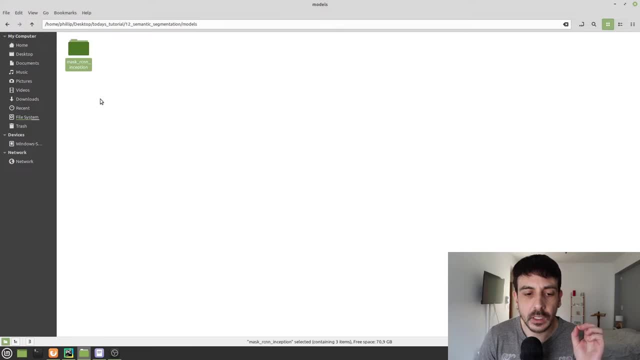 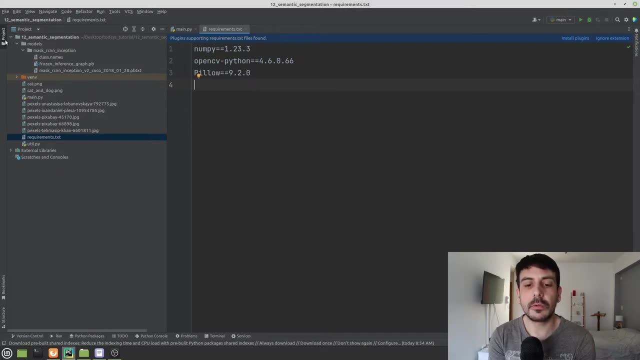 telling you exactly how to download these files. Now let me show you something else. If I go back to PyCharm, I'm going to show you another file which we are going to be using in this tutorial. This is an utils file which contains only one function, and this: 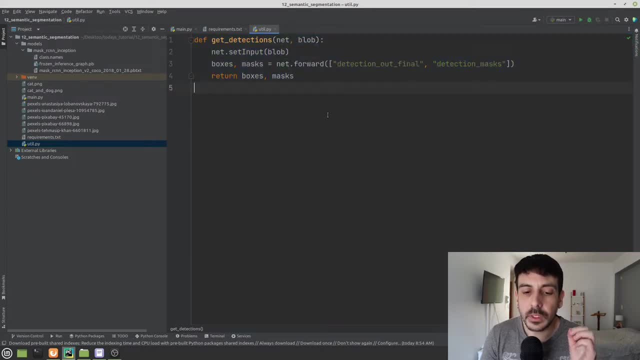 function is called getDetections. This is a function I created because it's going to make things much, much easier and much better for our process in this tutorial. It's going to make things much, much easier and that's why I created this function and I put this function into an. 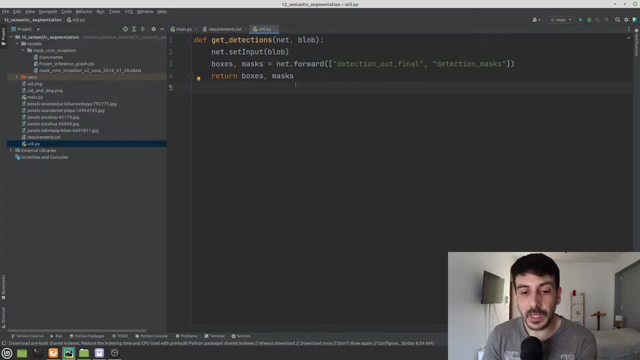 utils file. So we are going to be using this file and this function later on and I want to show you first this file, the utils file. Okay, so let's get started. and let's start with the first step, which is defining the paths. And what does it mean to define the paths? I'm going to show you. 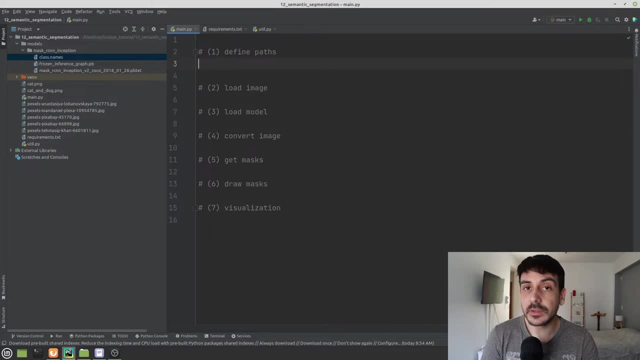 exactly what I mean. We are going to be using different files in today's tutorial. We are going to be loading an image, we are going to be loading a model, so the first thing we will need to do is to define what are the paths that are located. what's the file name for each one of these files? 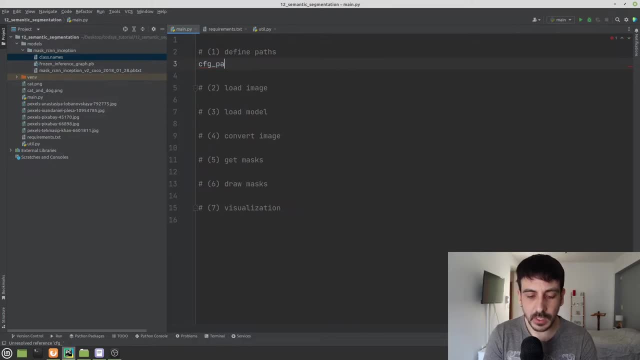 So what I'm going to do is to define a variable which is going to be called configPath, and this is: I'm going to import os first and this is going to be the path to our configuration file for our model, and this is going to be located in models: mask, rcn, inception and then the 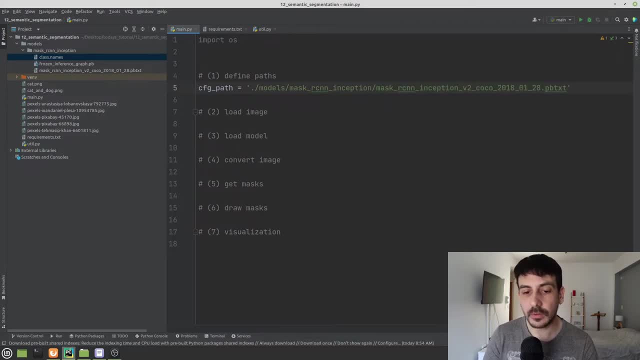 config file is mask one. Okay, so this is the location of the configuration file which we are going to be using today, and then I am going to define the weights path, another variable which is called weights path, and this is going to be a very similar file name, but it's going to be. 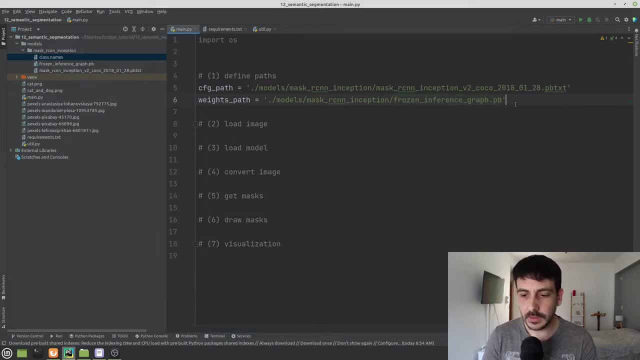 frozen inference graph: pb. Then I'm also defining class names, path and, And this is obviously the path, the file name of our classes, of our class names, which is located exactly here. Okay, and then the last thing I'm going to define is the. 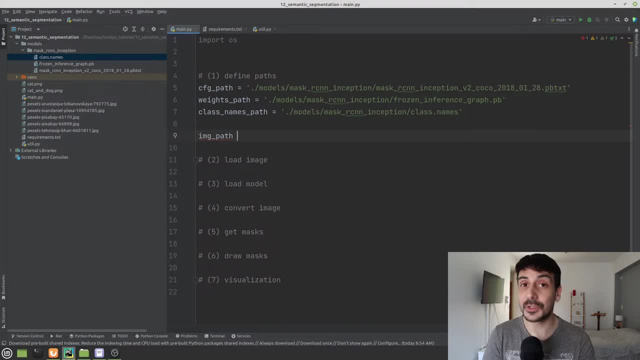 image path, which is the location of the image which we are going to be using today in order to test the performance of our model. So our image is going to be located in the current directory and it's. I have prepared many images for today's tutorial, but 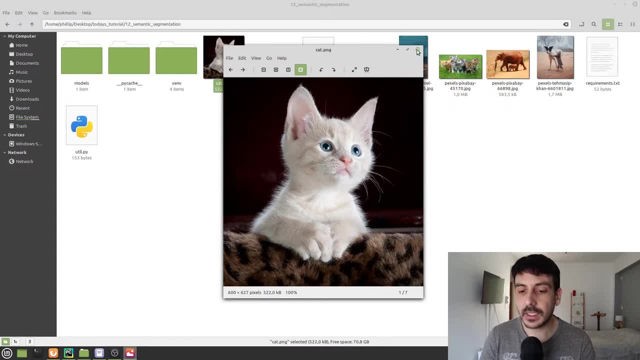 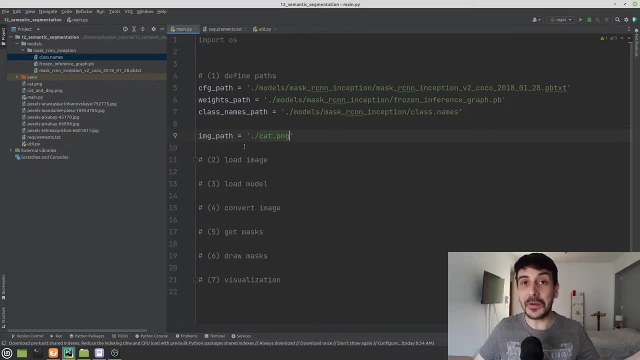 I think the one I'm going to use now is still this one, which is called cat png. So I am going to define cat png. Okay, and we have completed the first step in our process. You notice how simple this was. this is So. these are all the different variables. 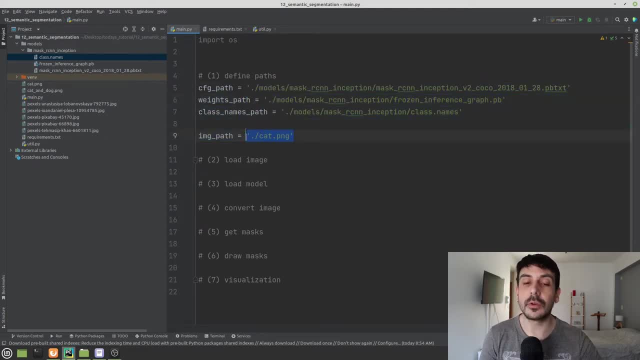 these are all the different file names which we need, we need to define in order to move forward with this process. Now, the next step in this process, in this sequence of steps, is going to be loading our image. So I am going to do something like image equal to cv2.img-read. 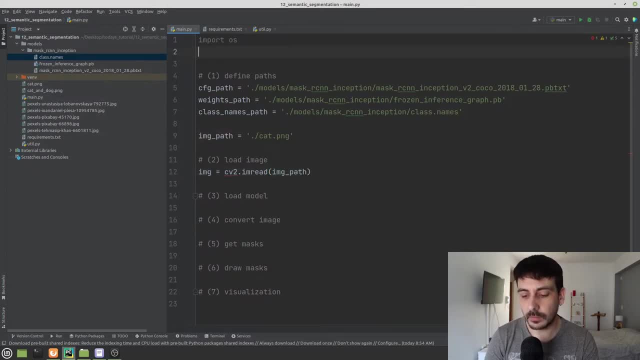 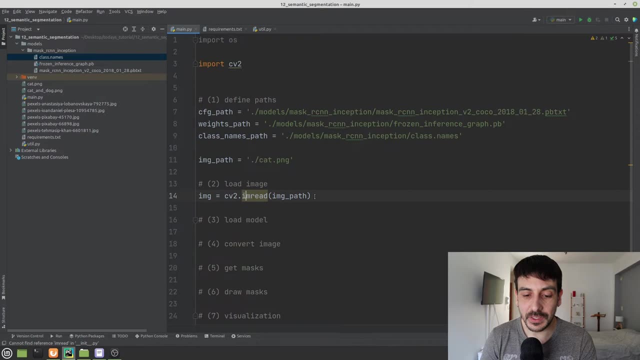 and then the location of my image, And obviously I need to import cv2, otherwise Python doesn't know what I'm talking about. And now I have imported cv2, so everything should work just fine. I'm going to make sure everything executes just fine and everything is perfect. What I'm going to do next is to load the. 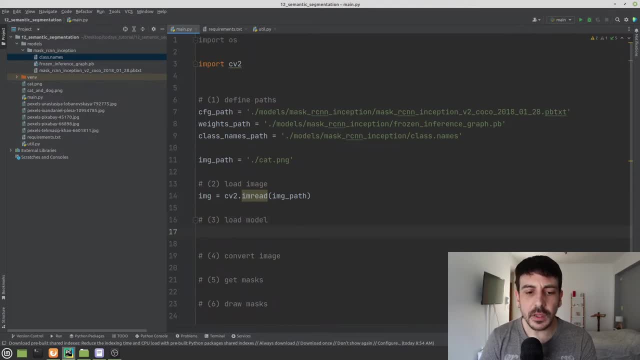 model which we are going to be using today, and this is a model which was trained using tensorflow. but the good thing about this tutorial, the good thing about this way to to to work with this model, is that we can load this model using opencv. we are going to call an opencv function in order to 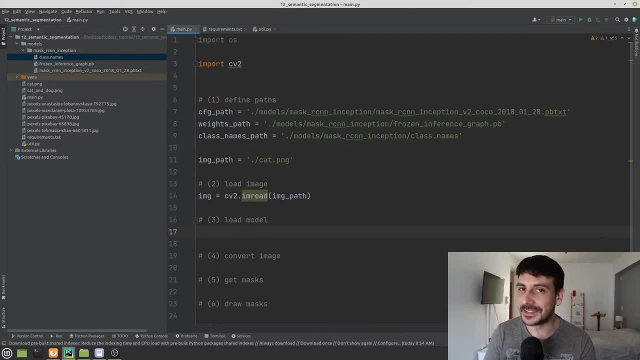 work with this model. wow, this is just amazing. this is amazing. so this is going to be something like cv2, dnn, um, something like read net from tensorflow, if i remember correctly, and the location of our configuration file and then the location of our weights file. okay, and this is. 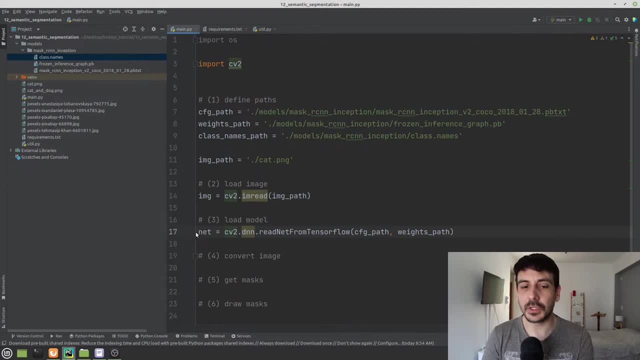 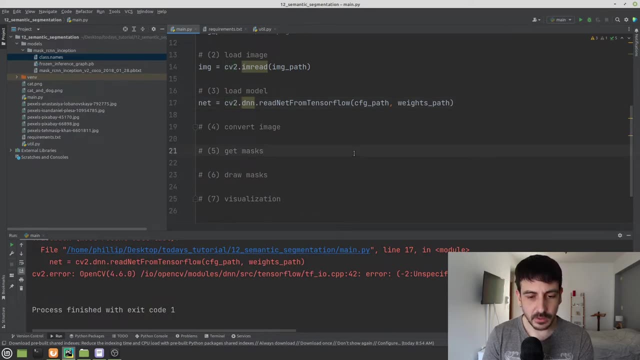 going to be equal to our model. so i'm going to call this object as net the see. if everything works, probably everything does not work properly. so let's see if i made a mistake. i see i have made a mistake. basically i have to input the weights file first. 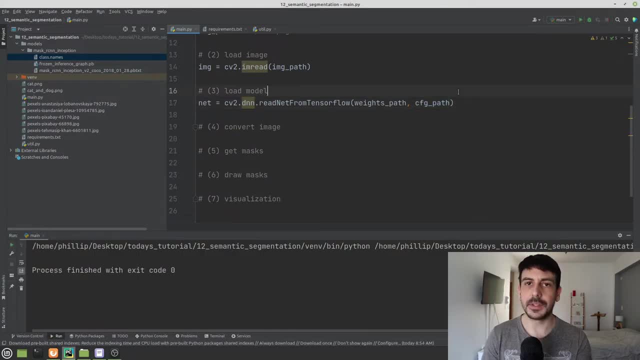 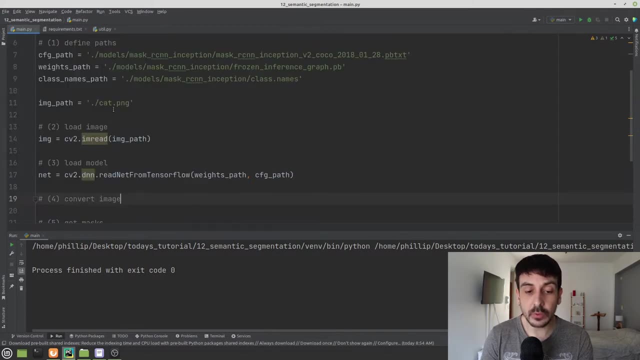 and then the configuration file. let's see now. everything works properly. so now let's move on. now we have um load an image which we are going to be using in order to test this tutorial. this is the image which we are going to be using. we have load our model, the. model which we are load to the softwareации which i stated, that when we build this новые model, there is noовой profile. weически we will see it on. so soon we will be using this, friends. we have load or model which we are going to be using the model using凉lyơng commandist, we are going to be 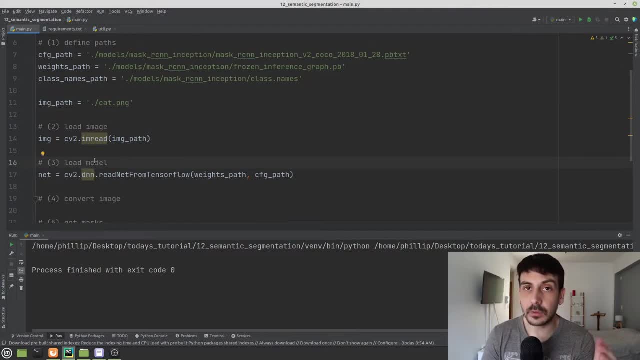 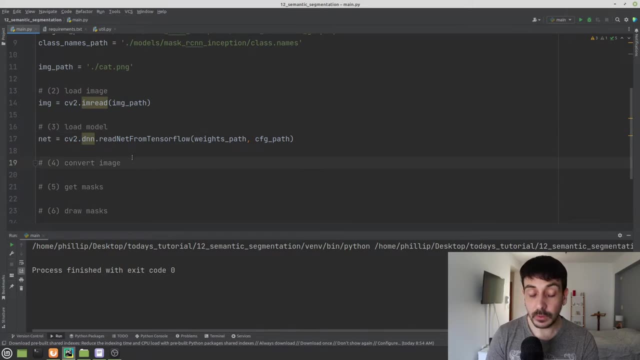 using that. it's gonna be in the server version in order to the project i have available, if I destroy the to use in order to get our detections, in order to get the masks, the, the detections from our semantic segmentation algorithm. and now what we have, what we need to do is to convert the image, to convert. 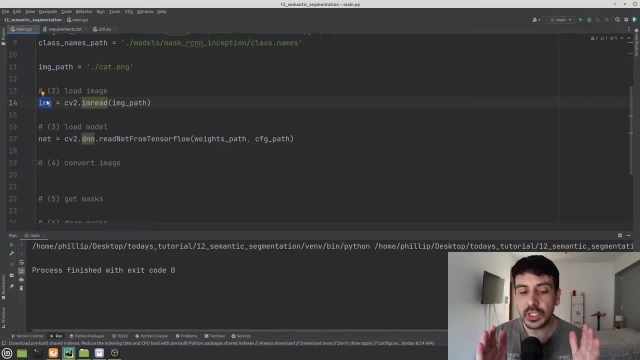 this image into another format, which is the format which we need in order to work with this model. remember that converting images or converting the data, it's a very common practice in computer vision or machine learning, so this is something that we usually do, very often, when working with. 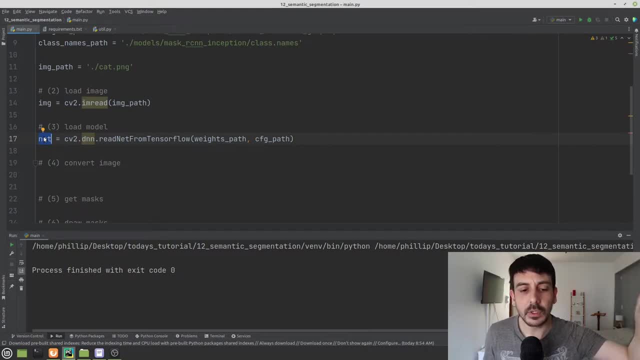 machine learning. usually we need to convert our data or images or whatever we are working with, among different representations. we need to convert our data through different representations. so in this case, we are going to define a new object which is going to be called blob, and this is going to be cv2 dnn. blob from image. 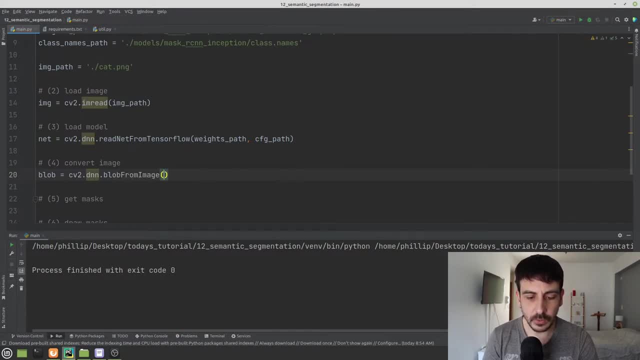 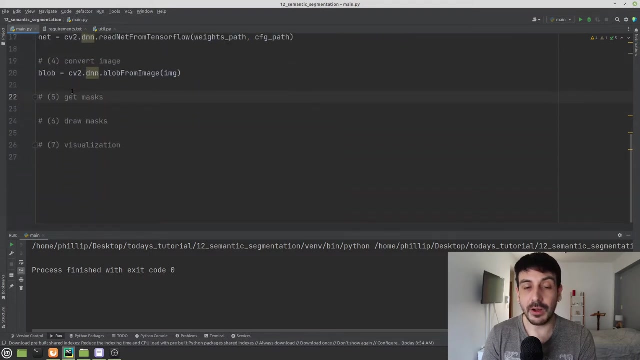 image and we need to input our image. okay, so this is basically how we convert our image into a blob and this is the type of object, the type of structure we are going to need in order to um, to input into our network, into our model. so you can see that we have completed four steps. 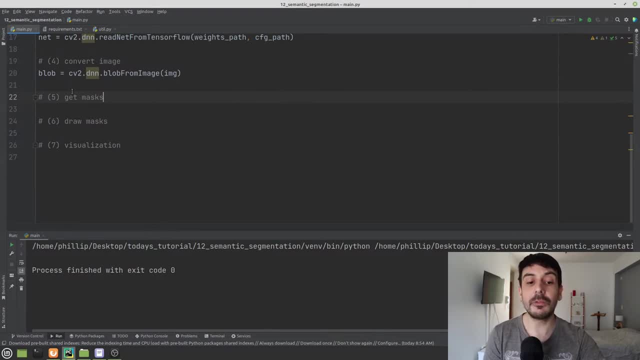 already. so we are pretty much there. we are halfway through, we are more than halfway through. you can see how fast we are moving forward. now the next step will be getting our masks. it's going to be getting our detections from the semantic segmentation. agree. so the way. 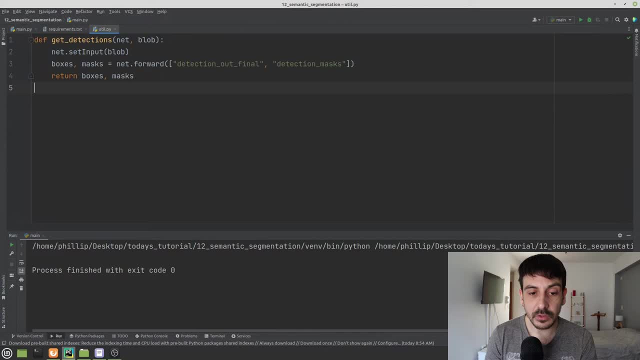 we are going to do this is by using the function i have defined in this utils file. so this is exactly why this function is going to be super, super useful. what i'm going to do is to import this function and the way i'm doing to do that. 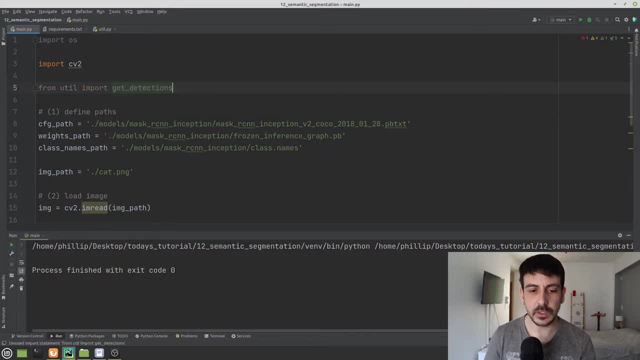 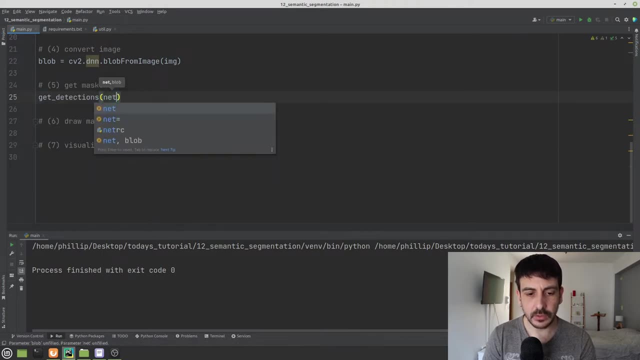 is from util import get detections. and now i am going to call this function by calling get detections. i'm going to input my model and also the blob i have just created, because if you notice the signature for this function, if you notice the structure for this function, 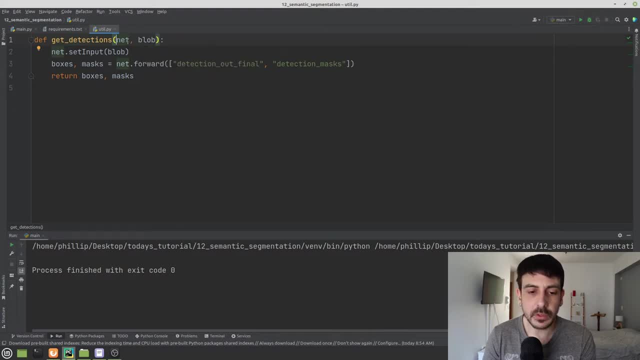 you realize that we need to input two variables, two parameters. one of them is the model which we are going to be using, and then the other one is the image converted into a blob and, by the way, this function. you notice that this is very, very simple. this is only a two lines function. 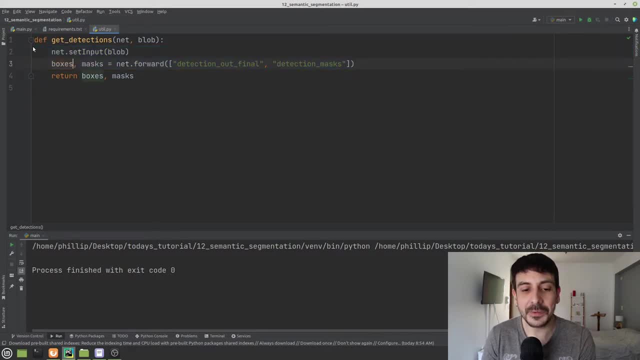 it's a two sentences long function and the only thing we are doing is to input this blob into the model. we are just setting this as our input and then we are getting the detections, getting the outputs from these two layers, from the detection out final, and the detection. 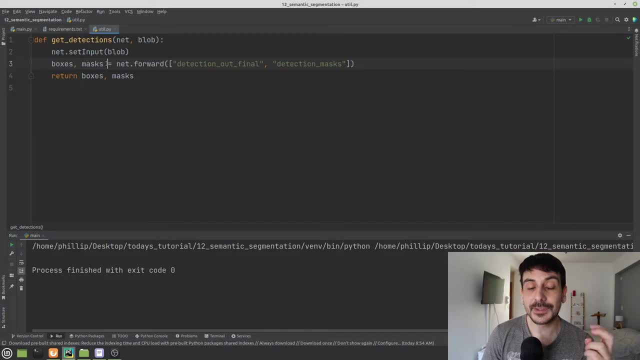 masks and the output from this function. it's two different objects. one of them is called boxes and the other one is masks, and you may guess that boxes is the bonding boxes for all the objects we are going to be detecting, and masks is all the masks, all the semantic segmentation masks. 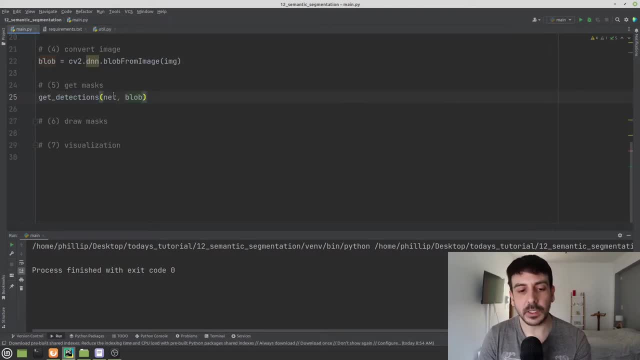 we are going to be detecting. okay, so let's get back to our main code. and now we are going to say: this is going to be equal to boxes and masks, and that's it. now we have completed five steps in our process. so we are moving super, super fast. and this is going super, super well. let me see if everything runs smoothly. 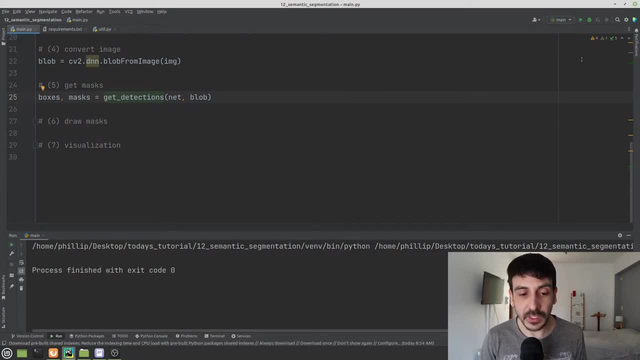 because this is something we have to check once in a while when we are coding. and yes, everything runs smoothly. i don't have any error, so we can continue now. the next step, drawing the masks, is going to be the most complete, complex part of this project. this is the step in which we are going to spend most of our 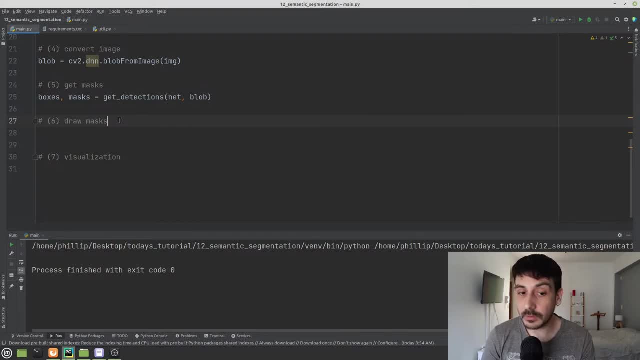 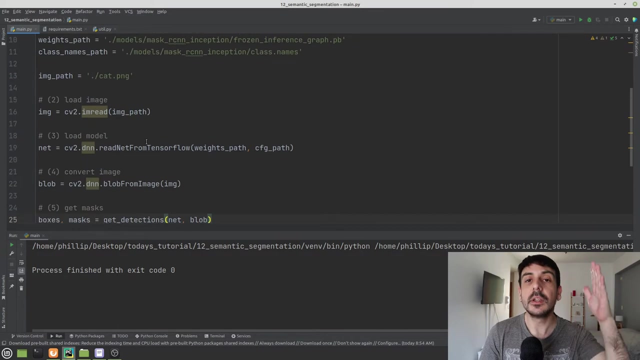 time, because this is going to be. it's not going to be hard. i'm going to walk, i'm going to be with you. like the entire time, this is not going to be hard or complex at all, but if we compare the complexity from drawing the masks against the complexity of each one of these steps, you are 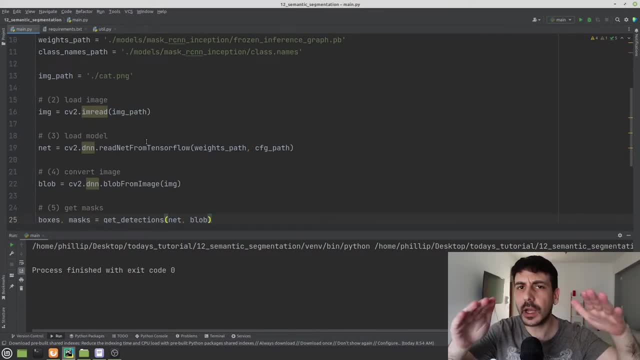 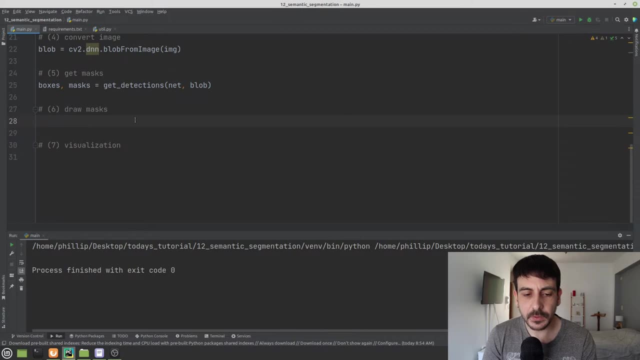 going to know. this is slightly more complex, but don't worry, i'm going to be here and going to explain absolutely everything. everything I do so in order to draw the masks. the first thing I'm going to do is to define another variable, which is going to be called empty image. 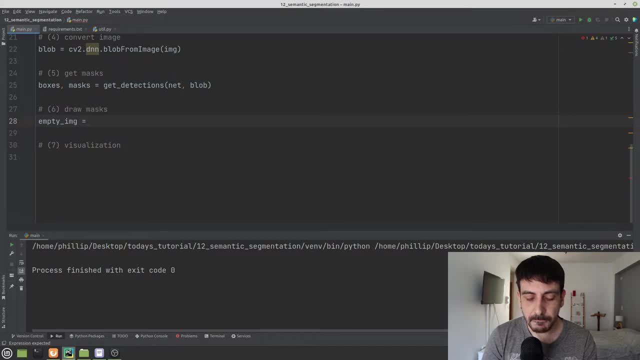 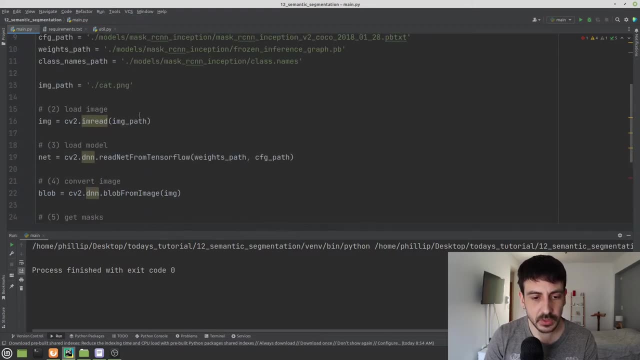 something like this, and this is going to be an empty image. so I'm going to just create something like MP zeros and the size of my image. and the size of my image is going to be image dot shape. this is equal to HW and the number of 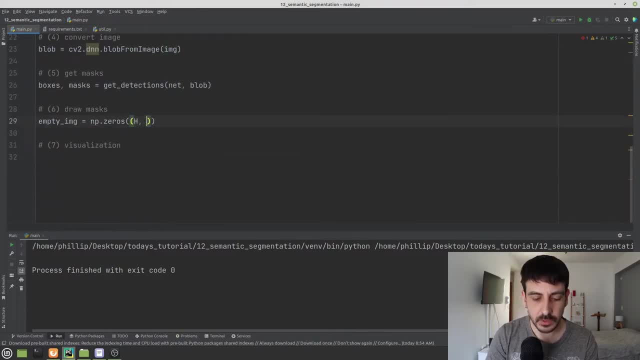 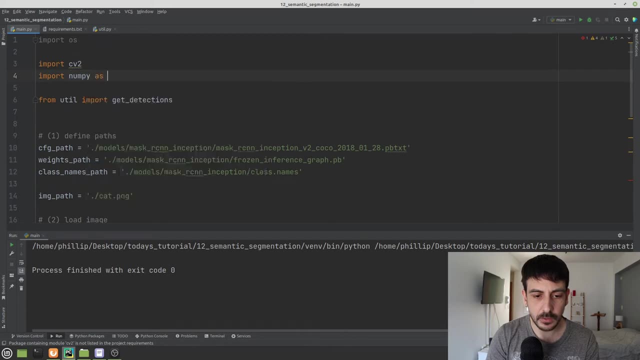 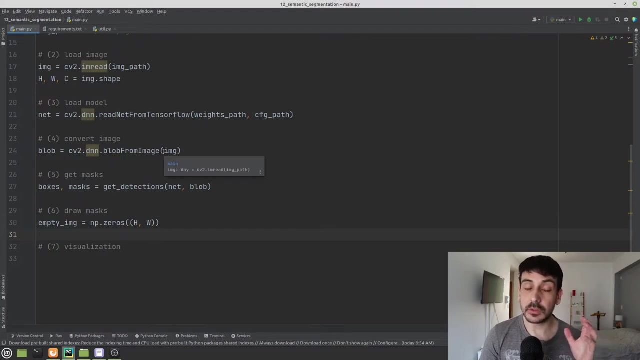 channels. okay, and now H and W, and that's going to be enough. I need to import numpy as MP or what is not going to work, and that's it. so this is the first step: defining an empty image, which is an animation I'm going to use in order to 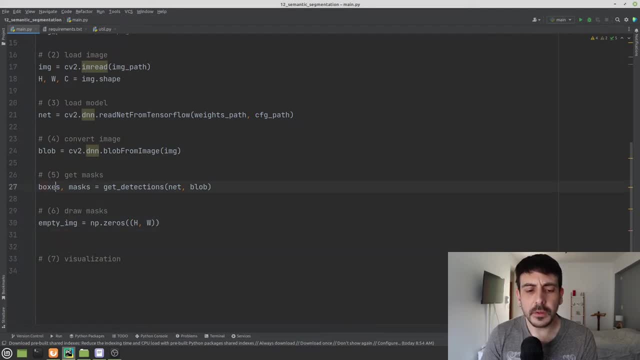 move forward with my process. so we have the technique that I'm going to use in order to move forward with my process. so we have the technique that I'm going to use in order to move forward with my process. so we have the technique that I'm going to use in order to move forward with my process. so we have the detected many boxes and many masks. 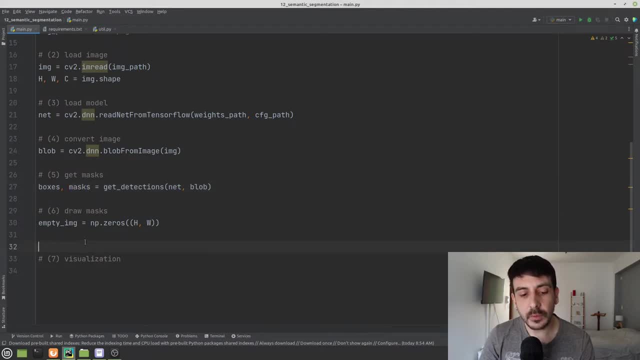 detected many boxes and many masks, detected many boxes and many masks. eventually, we have detected many, many, eventually, we have detected many, many, eventually, we have detected many, many objects. so the first thing we need to do objects. so the first thing we need to do objects. so the first thing we need to do is to iterate in all the objects we have. 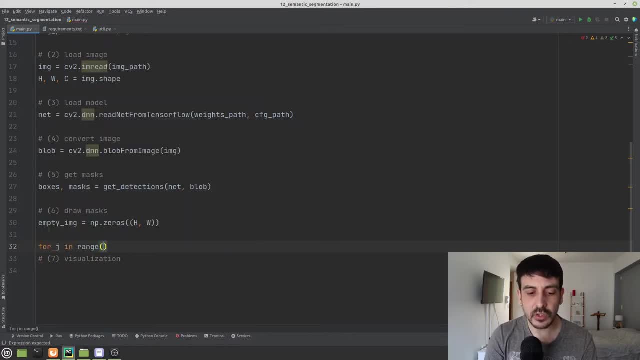 is to iterate in all the objects we have, is to iterate in all the objects we have detected. so I'm going to do something detected. so I'm going to do something detected. so I'm going to do something like 4j in range, like 4j in range. 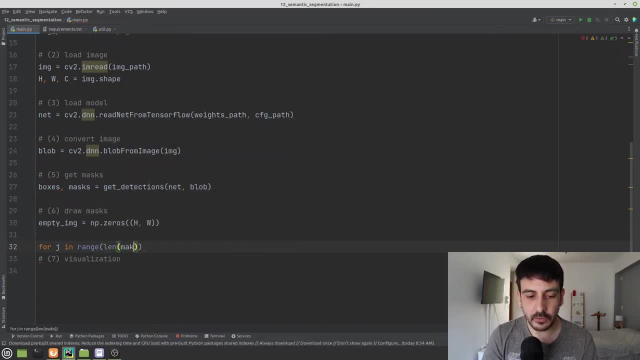 like 4j in range, len, and this is going to be the length of len and this is going to be the length of len and this is going to be the length of my masks. right, I'm going to iterate in all the objects i got as our detections. so each one of these iterations is going to be one of four. 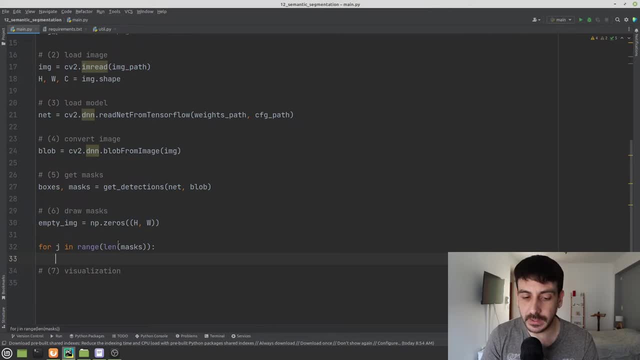 detections, one of four masks, one of the objects we have detected. so the first thing i'm going to do is to unwrap these two objects and i'm going to say: my bounding box is equal to boxes j. let me write it first, and then i will explain it, and then my mask will be something like: 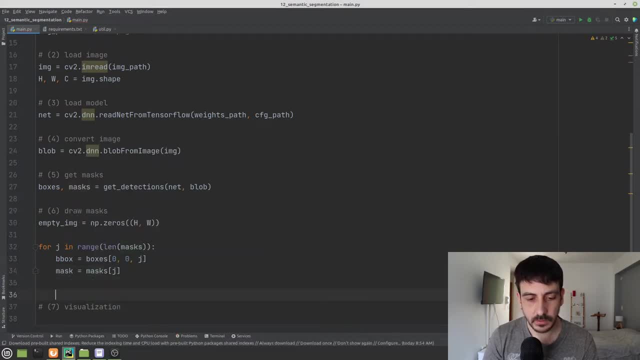 mask j. okay, and then i'm going to write a few, a couple of more sentences, and i will explain everything in just a minute. i'm going to say that my class id is equal to bonding box one, and then i'm going to say my score is equal to bounding box two. okay, what am i doing here? i am iterating in all the different 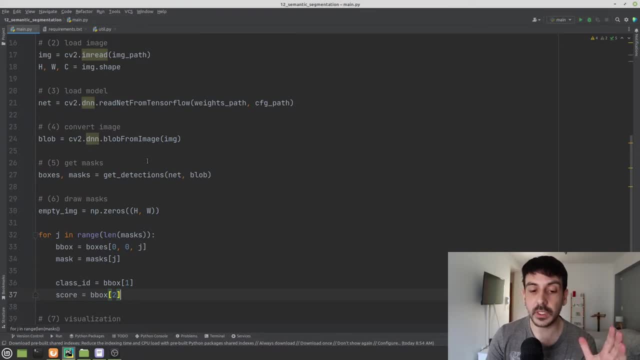 objects. i got from this model once i i i input my image into this model and i got a lot of detections. now i am iterating through each one of these detections, through each one of these objects and through each one of these detections, i am just, uh, getting some information. i am just 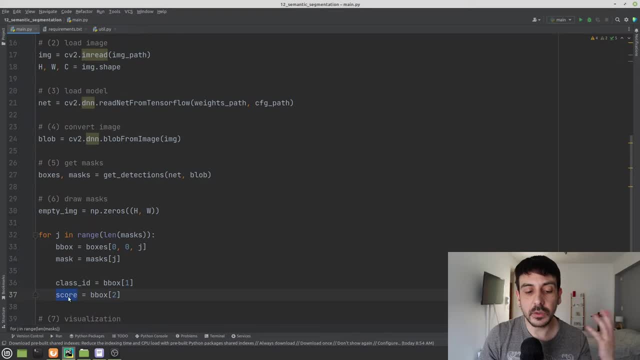 getting this parameter, which is class id. i am getting this other parameter, which is score, and now i'm going to do other things with it, but so far, the the most important thing you should keep, the most important thing you should know about these steps is that i am iterating through. 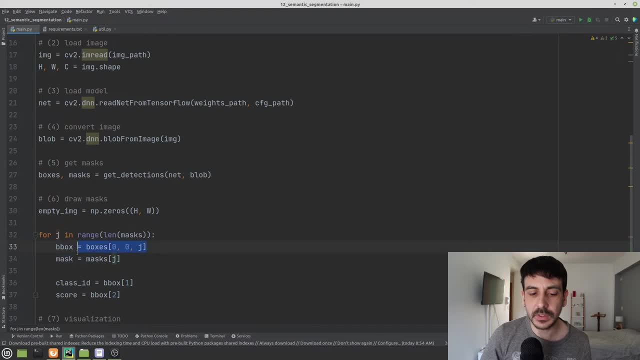 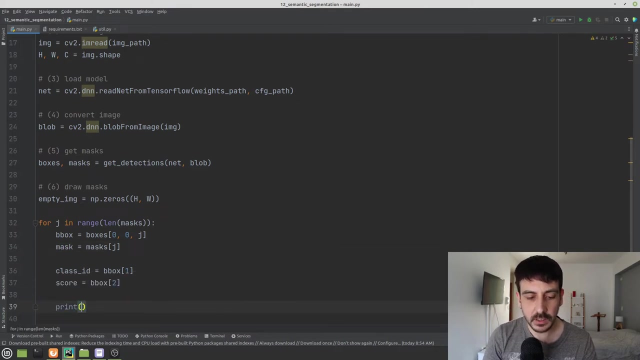 each one of my boxes, each one of my bounding boxes and through each one of my masks. i'm just iterating now. something that's very important is: let's see what's the shape of this box and this mask. so i'm going to print something like bondingboxshape and print maskshape and 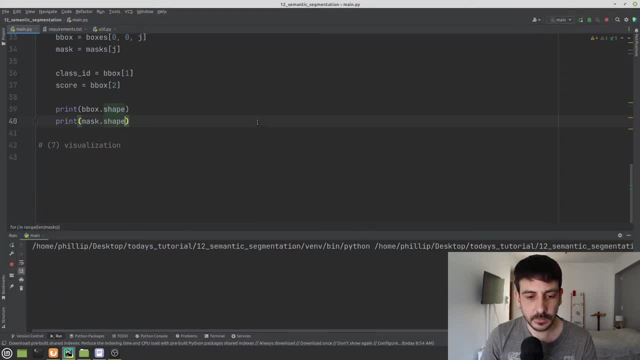 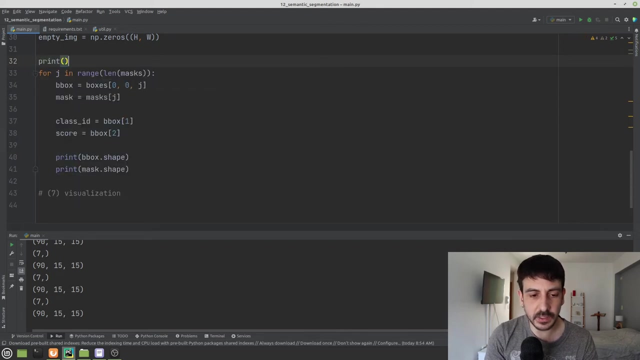 let's see what happens. i wait a couple of seconds and i get many, many outputs because we have many, many objects. so maybe the best thing is to ask how many objects we got. so let's print something like this: let's see how many objects we have detected using this. 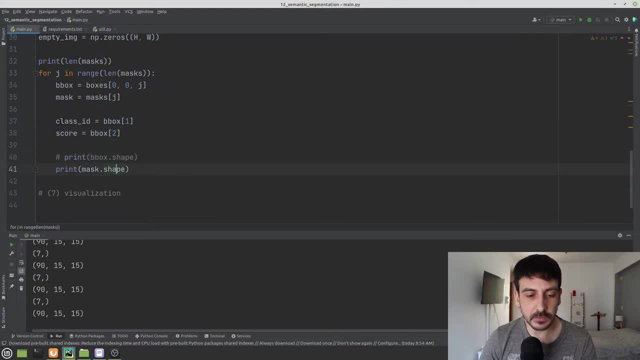 algorithm. in this image i have inputs, so i'm going to comment this for now. and we have detected 100 objects. we have 100 objects in which we are iterating. so something important is that if i show you the image again, you can see it's only an image of a. 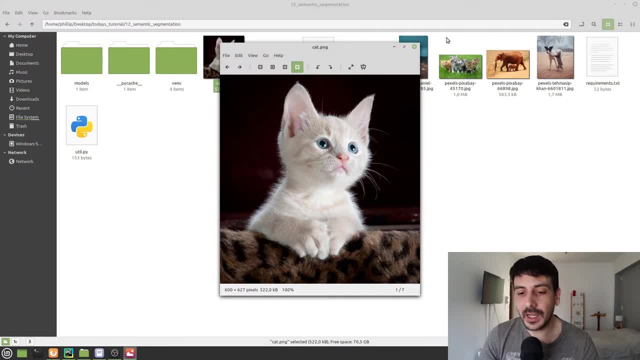 cat, so there are not so many objects at all. and the third thing we will, we will need to do, is to do some cleaning or to do some filtering in order to keep only the objects we are interested in. in this case, we should be getting only one object, because we can see the image and it's only one cat. so what? 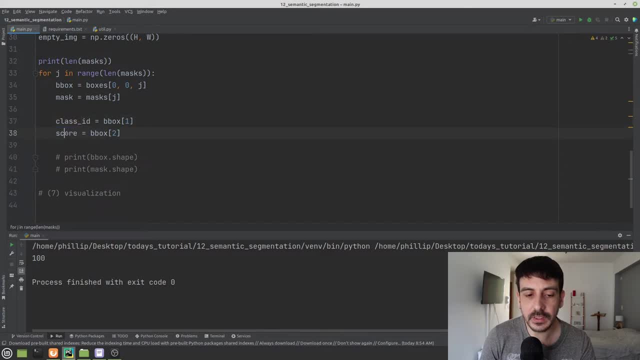 i am going to do is, now that we have the class id and we also have the score, i am going to do something like this: i'm going to continue doing my my process and continue doing my my stuff only if the score is greater than um, something like a threshold detection. 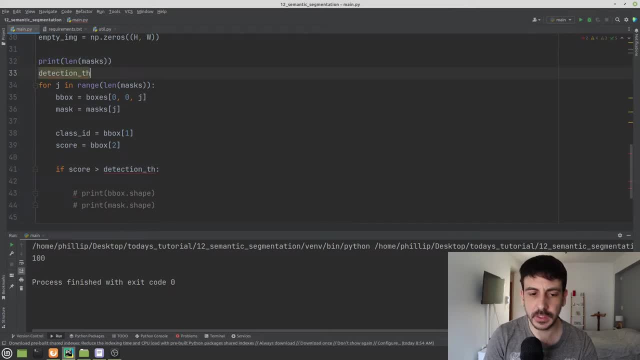 threshold, and i am going to define this detection threshold in 0.5. so this is going to be my detection threshold. once i detected an object, i am going to check what's the score for this detection. how confident is our model about this being in fact an object? and once i got this number, 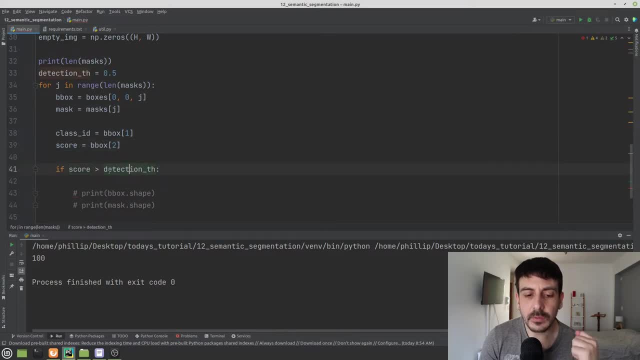 i am going to see if this number is greater than or detection threshold, which i have said in 0.5. remember that our score or confidence value, it's always going to be a number, a float number between 0 and 1.. so if our model is not confident at all, for in in the detection if it says 0.5. 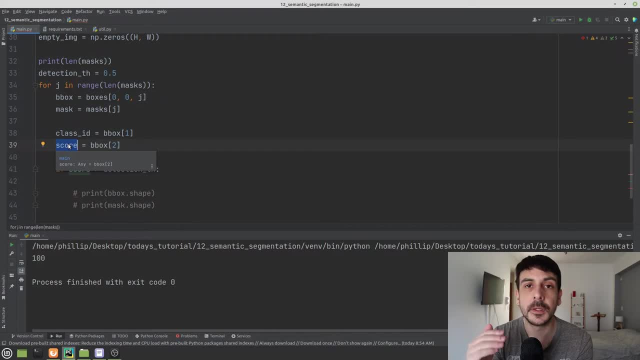 then it's going to be 0.5. so if our model is not confident at all for in in the detection, if it says it's very um, if it's not confident at all, it's going to be something that's closer to zero. and if it's super, super confident and it's super convinced that this detection is an, 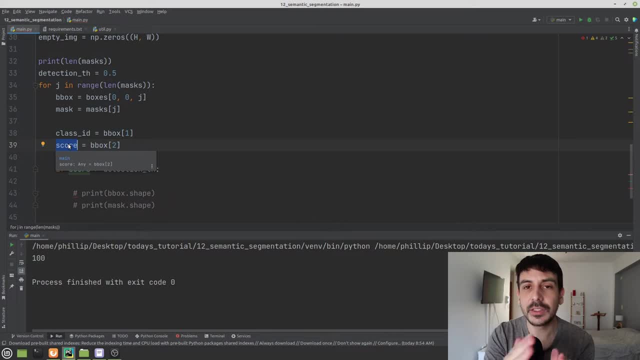 object and that it's a very clear object, and so on. it's going to be a number that's closer to one. so the way we are going to do some filtering in all these 100 detections is by asking e4 confidence value is greater than 0.5. 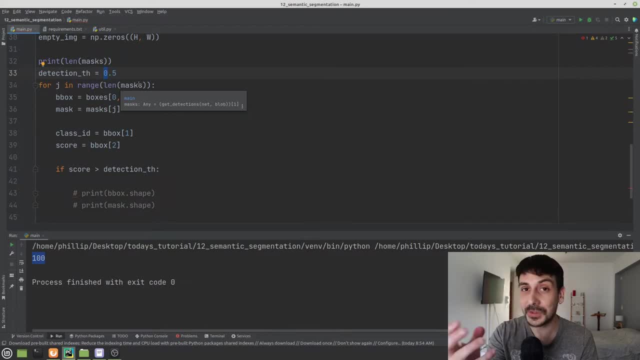 if it's greater than 0.5, then we are going to consider this object and we are going to do some more computation and some, some more stuff. but if it's not, then we are not going to consider this at all. so now i'm going to do exactly the same, but i am going to print only in this case, if the 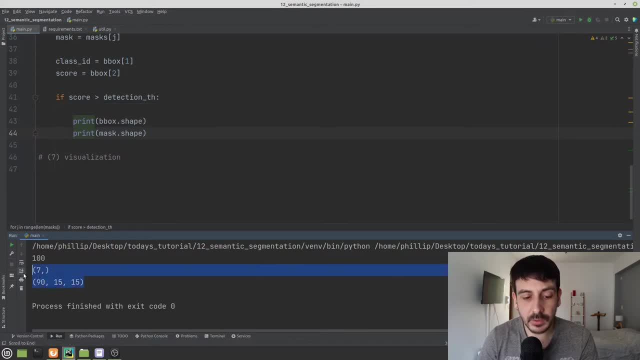 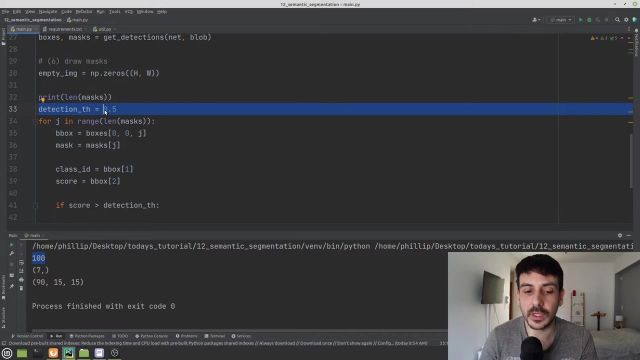 score is greater than detection threshold, and you can see that now i am just printing two objects to arise. so this was so. this means that from all 100 objects, only one of them meets this criteria. only one of them was detected with a confidence value greater than 0.5. and if i go back to the 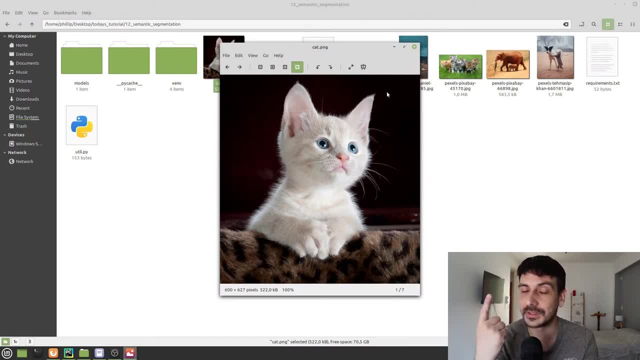 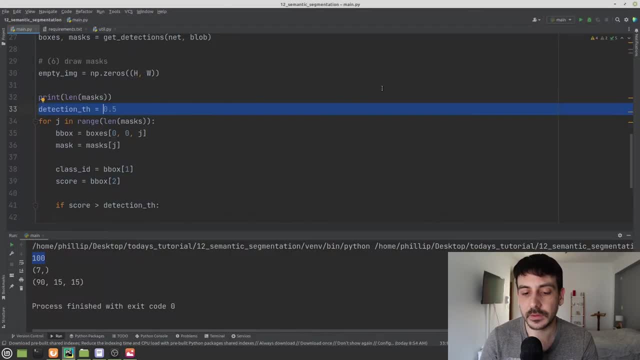 image. it makes perfect sense, because there's only one object, there's only one cut, so only one object should have been detected with a very high confidence. so let's get back to these results, but to this arise and you can see that we have two arrays. one of them is length. 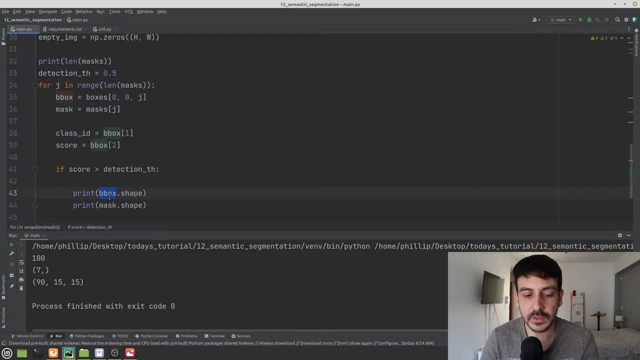 seven. so the bounding box is only a list of seven elements. and then the mask is something like an ampere array of dimensions 15 times 15, and it has 90 different um indexes. it has it's something like 90 different images of this size, 15 times 15. now about the bounding box. 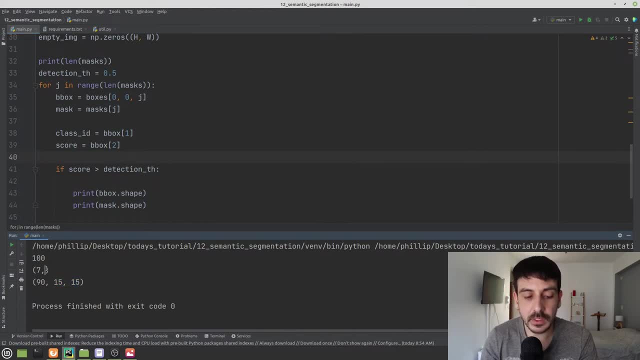 these seven locations. this size, it's exactly the size we need in order to unwrap all the information of this bounding box. we have already unwrapped the class id. this means what's the class that was detected in this bounding box. also, we have unwrapped the score. 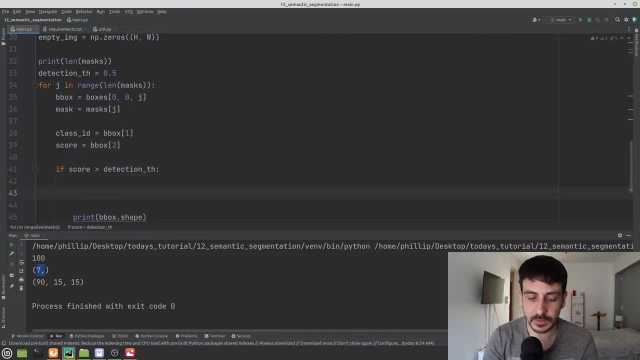 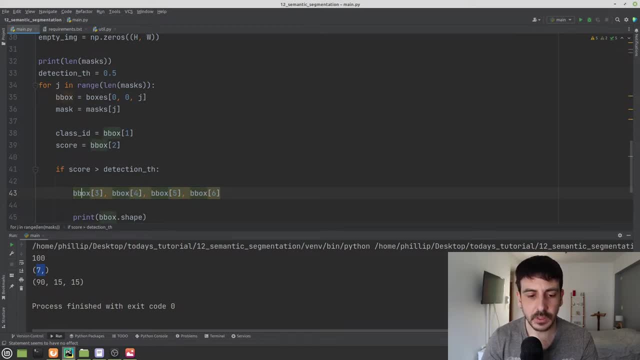 we are going to do something like this. we are going to do something like this. we are going to do something like: this element is actually the last element and we are going to say: this is equal to x1, y1, x2, y2, and we are going to say that this is. we're going to say that this is equal to this, so x1 is going. 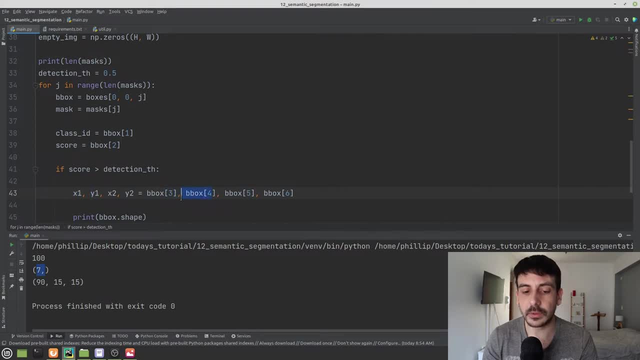 to be equal to bounding box 3, y1 is going to be equal to bounding box 4, and so on: x2 equal to this number, and then y2 equal to this other number. so we have defined these four numbers, and now let me show you how these numbers look like. i'm just going to print these four numbers. 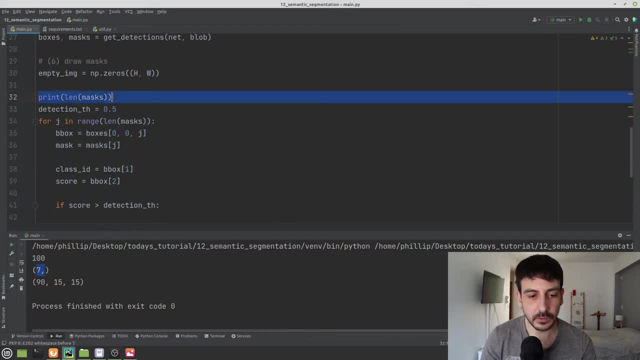 let's take it one step at a time. i'm going to remove this print because i don't need it anymore and i'm going to press play again. so this is the output from our print. you can see that this is our. these are the four numbers we have just print. 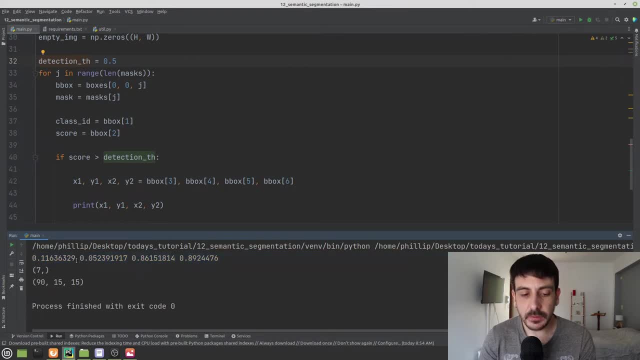 And you can see that the location of our object is given in relative numbers. We have four float numbers and each one of these numbers is one of the coordinates of this object. Now, we don't really want relative numbers, but we want absolute numbers. 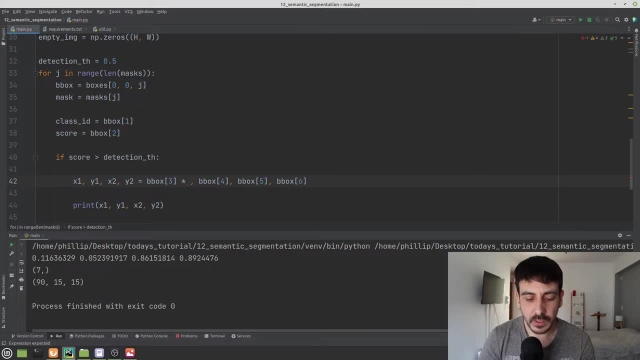 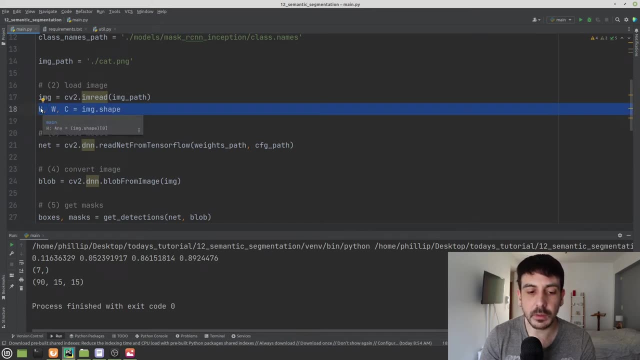 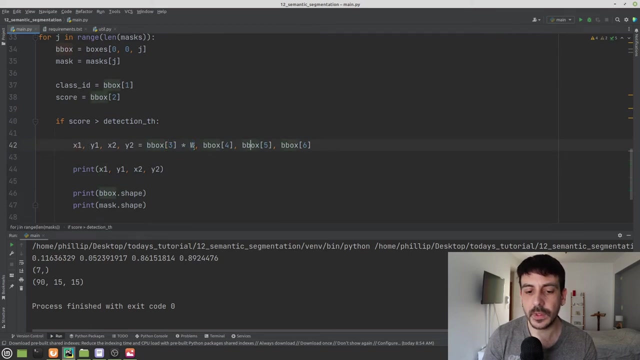 So what I am going to do now is to multiply each one of these numbers times the height and the width of our image. Right, I'm going to multiply these numbers times H and times W. So the X1 and X2 I'm going to multiply by W, because that's the width of our image. 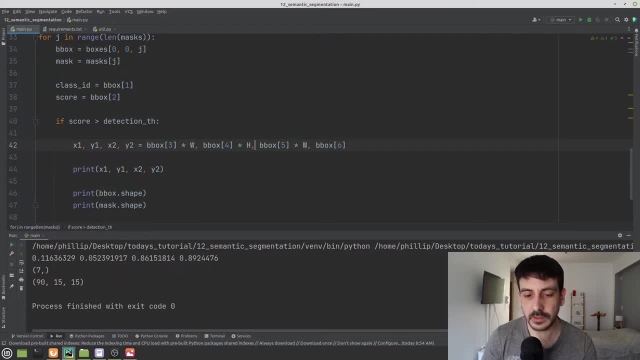 And then the Y1 and Y2. I'm going to multiply it by H And something else I'm going to do, and I'm going to do everything on the same sentence, on the same line. So please focus, Please pay attention, because otherwise this may be a little confusing. 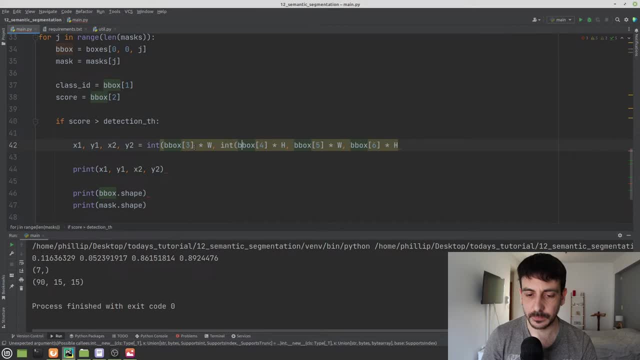 I'm going to cast Each one of these numbers as an integer, So I'm going to do something like this And then something like this. OK, The reason I'm doing everything in the same line is just because I like it. It's just because I really like one liners. 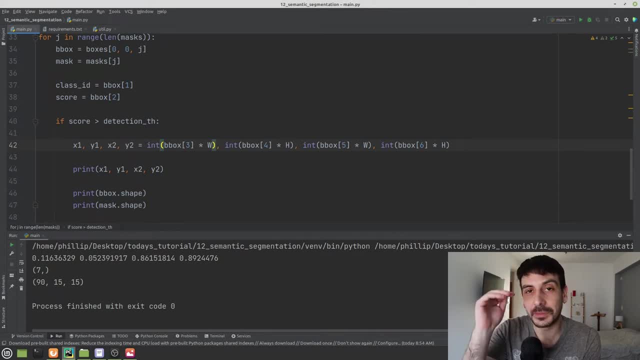 And I think that we can do this in many, many different lines, many different sentences, But we're not really doing anything. We're not really doing any complex project. It's just defining these variables and then assigning these variables to the bounding box coordinates. 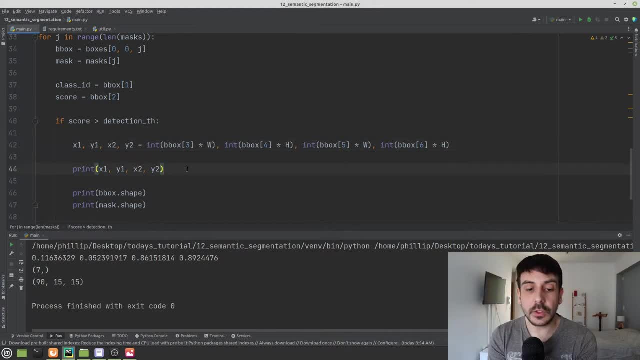 So I think it's going to be cleaner if I do it in one line. So now let's continue. I have unwrapped the bounding box and now we have all the coordinates for our bounding box. What I am going to do next is to explain why this looks the way it does. 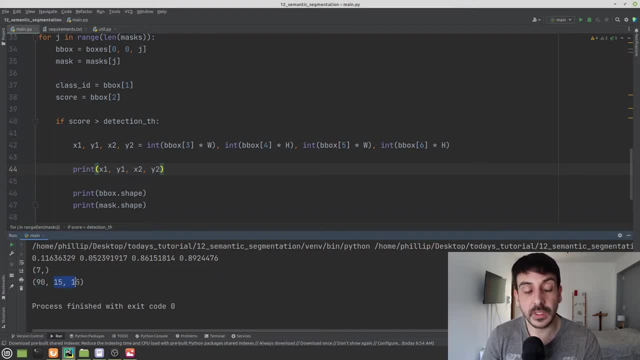 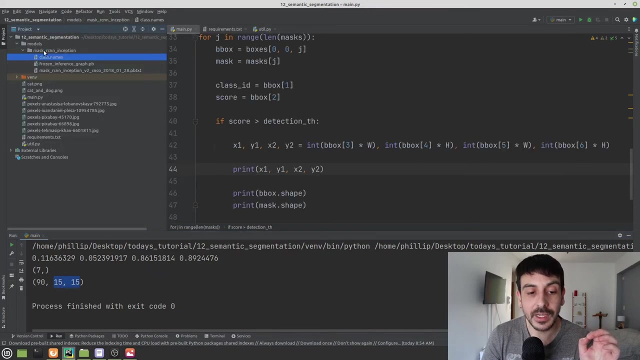 Why we have 90 different images of this size, 15 times 15.. The reason for that is that the number 19 is because each one of these images is going to be the mask we have detected by for each one of four classes. 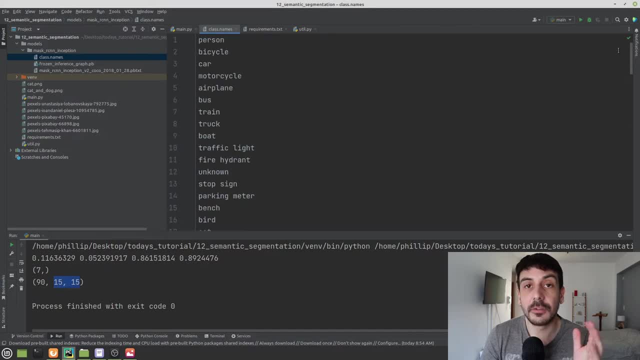 If I show you back the classesnames file- this is a file which contains all the classes we can detect using this model- You are going to see we have exactly 90 classes. So this means that each one of these elements, Each, Each one of these very small images are one of four classes. 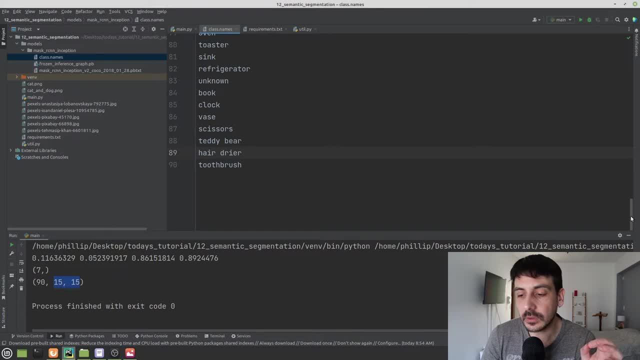 So if I, if I check the first element is going to give me a mask which is going to be for the person, And if I show you that, if I check the next elements, you're going to be the one for the bicycle, and then for the car, and then for the motorcycle, and so on. 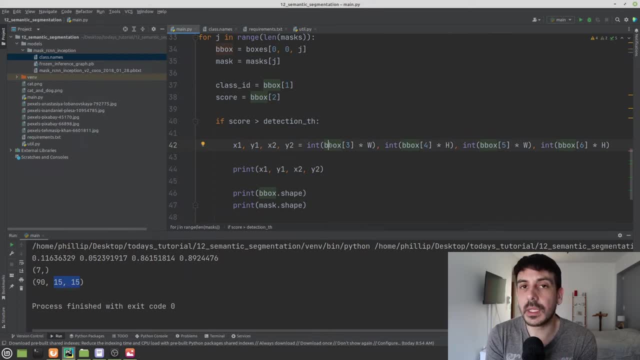 But they- not all of these bounding boxes- make sense. The only one that's going to be the only one, So that's going to make sense is the one that the belongs to the class We have detected. this is the class we have detected. 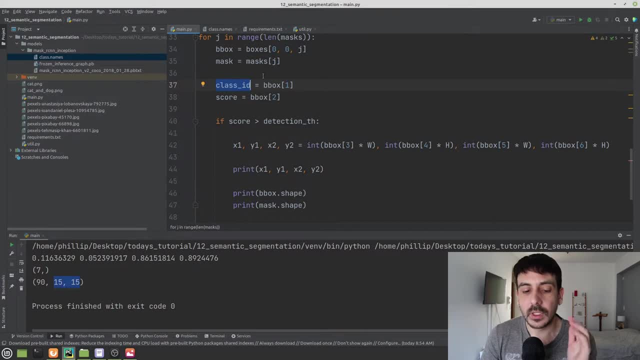 So this is the only class we should care about. So what I am going to do is to say something like: I can delete this for now. I'm going to say: mask, equal mask in class 80. from these 90 objects, I am going to keep only 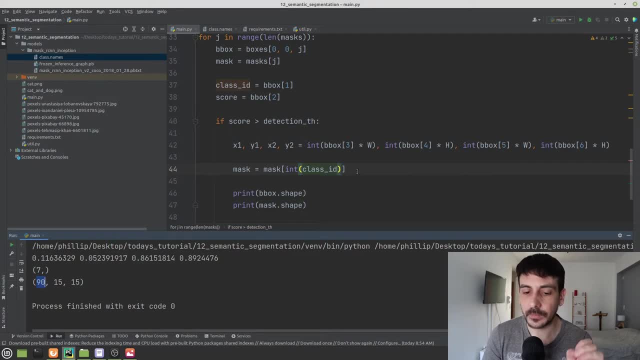 The one that we have detected, Only the one for class ID. Now I'm going to print mask dot shape again. I'm not going to print box dot shape anymore because I don't need it. And I see that now we have a shape of 15 times 15.. 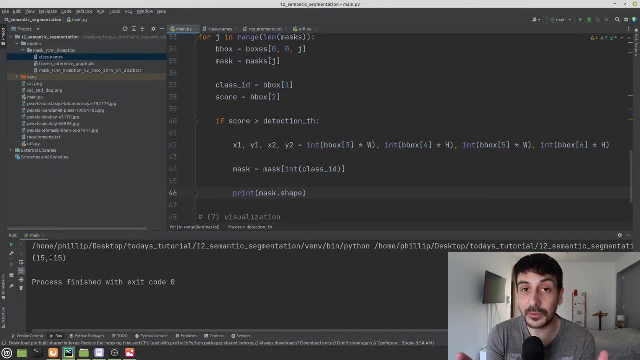 So these objects we are printing now, This is the mask of our object, This is the mask of the object we have detected. We have 90, 90 masks. We have the mask for each one of four objects in our classes dot names file. 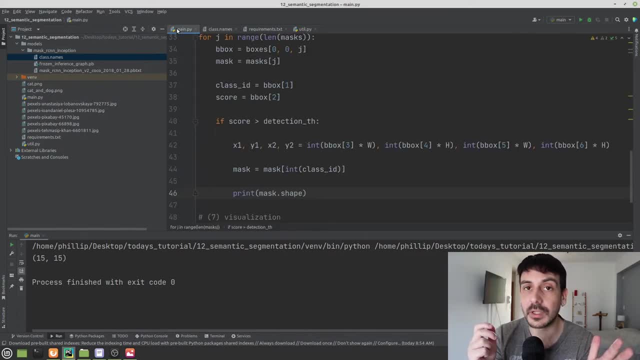 But now we are just keeping the one of the object we are interested about, Right, This is the way we are going to do it. This is the only mask that makes sense in this case. So this is what we are going to do. 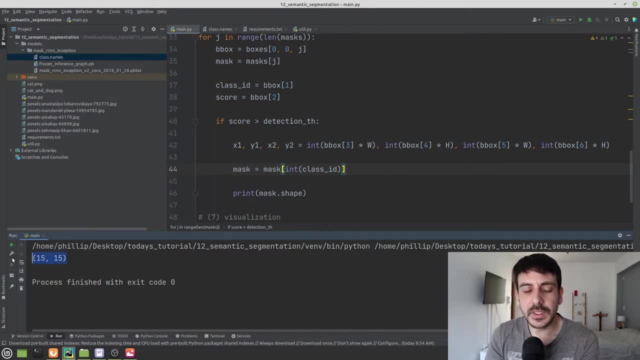 And something that you may wonder is: hey, Felipe, So why is this this size? Why is this 15 times 15?? I mean, it's a very small size. It doesn't really make any sense, And I am going to tell you that that's the way it works. 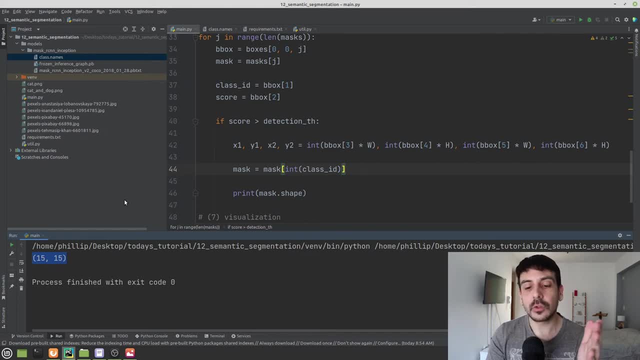 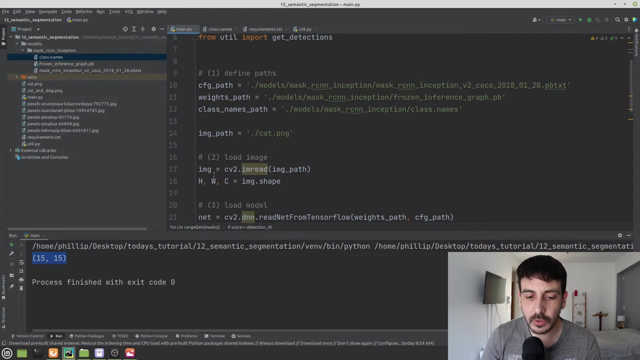 And that's going to be the mask we are getting from this model. So what do we need to do in order to get, in order to resize, or imagine in order to get something of a different size is going to be something like this. Let me print also the shape of our original image. 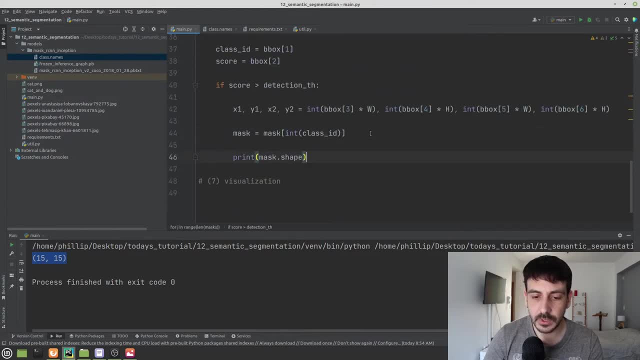 I'm going to print these two numbers. So let me show you first What's the size of our original image. and you can see that the size of our original image is 627 times 600. So we have to take this 15 times 15 to something that's more close to this number. 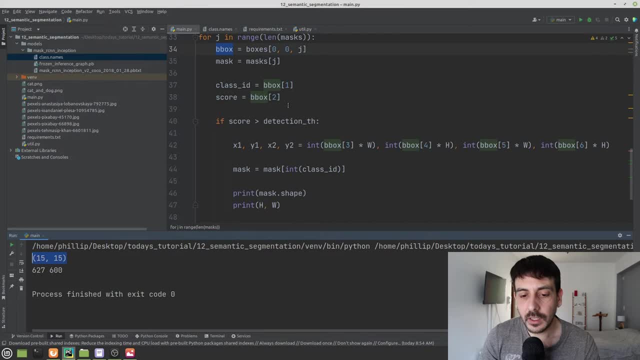 Let me show you something, and it's going to be a little more clear. What I'm going to do is to define a rectangle and I'm going to show you first how this bonding box looks like on our image. I'm going to input my image, then I'm going to input two points. 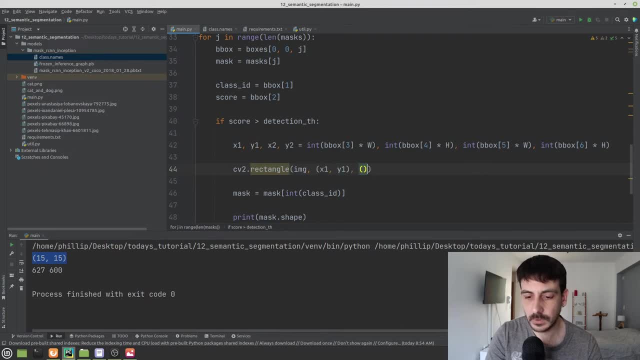 One of them is going to be this one, and the other one is going to be this one. This is going to be a green rectangle, and the thickness for this rectangle is going to be five. Okay, so this is image, And now, very quickly, 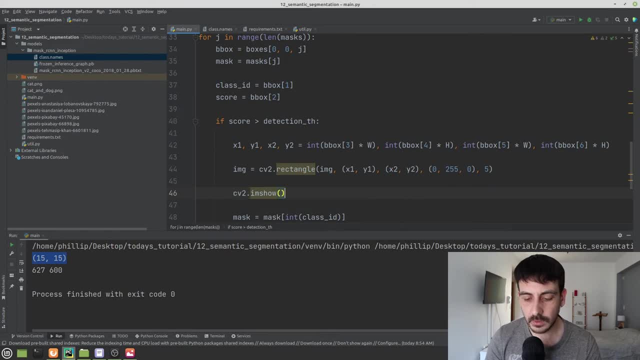 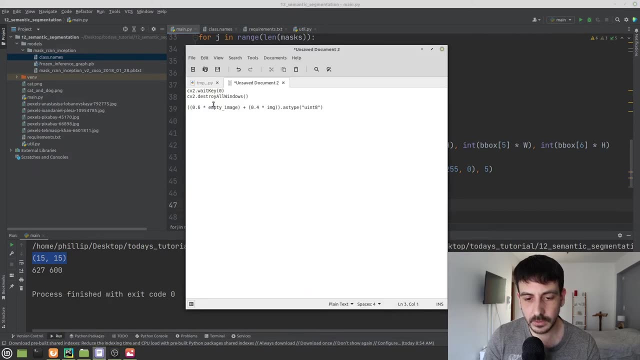 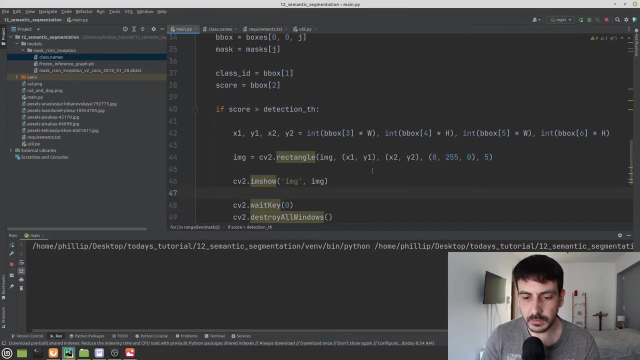 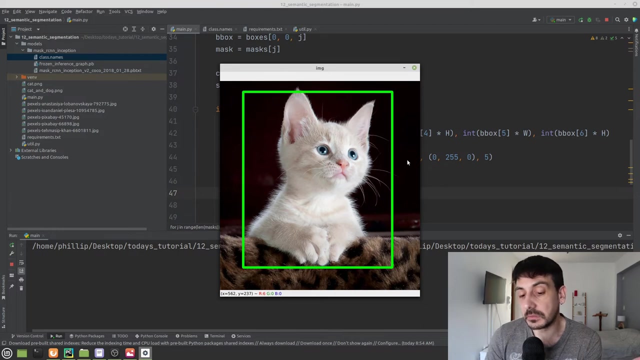 Very quickly. Let me call cv2- imshow image, and then let me copy and paste this number: Okay, these two lines. Let me press play. Let me see if this works properly. So this is the bounding box we have detected, This is the object that you can see. everything works perfectly. 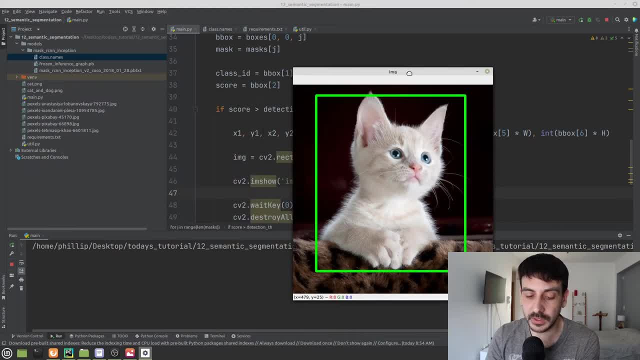 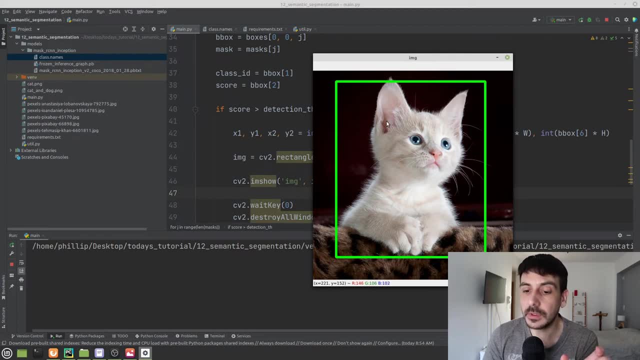 This is exactly the object we have detected. This is working super super perfect, perfectly, And what we are going to do now is to resize the 15 times 15 to match this bounding box, to match the size of this bonding box. That's what we are going to do. 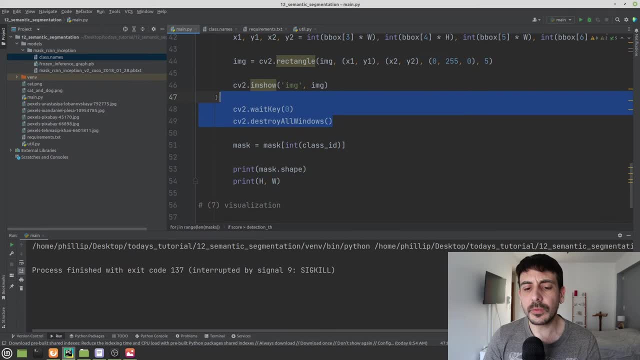 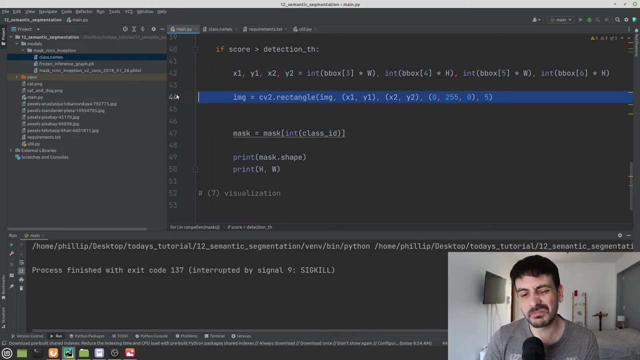 So let me move forward and let me remove this in these sentences for now, because we are not going to need it, And let me remove the bounding box as well, because we are not going to need it anymore. This tutorial is about semantic segmentation, So we are going to focus on the mask, only on the mask. 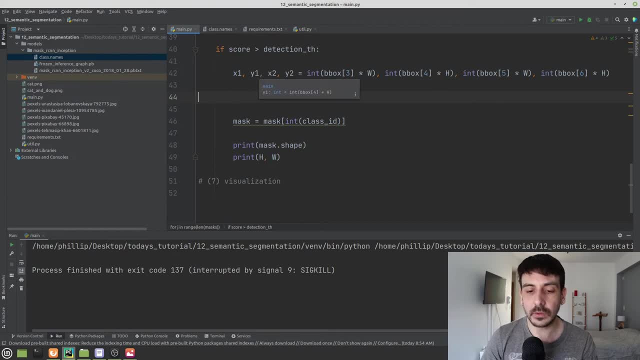 We are not going to focus on the bounding box. So what I am going to do now that we have our mask is to resize our mask, And this is going to be resize. I going to input my image mask. This is an equal. 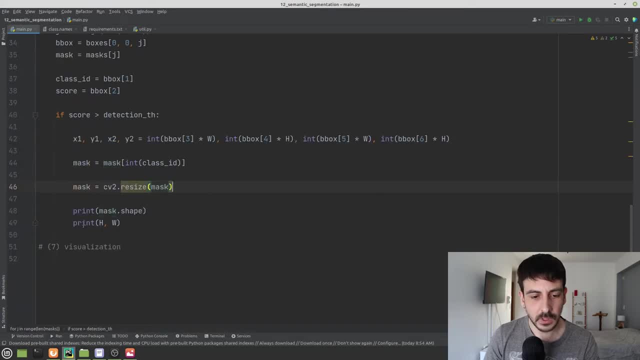 And let me close this one and this one. And this The new size is going to be: if I remember correctly the order, it was H. sorry, The new size is going to be, if I remember correctly, the order, X2 minus X1.. 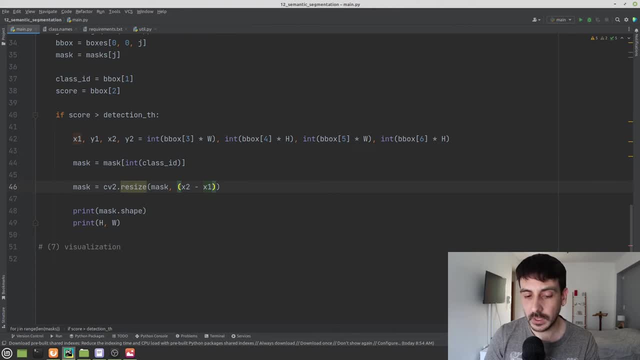 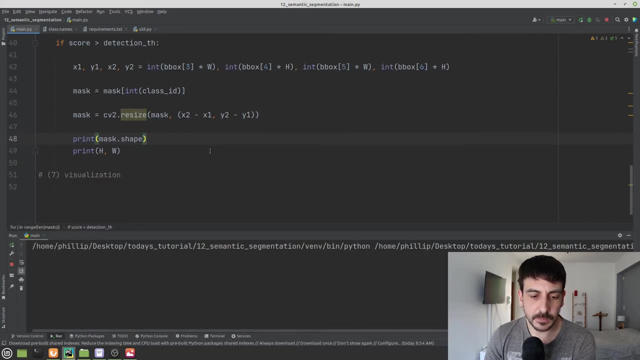 Remember we want to take everything to the size of our bounding box, and then Y2 minus Y1.. Right, And if I press play, you can see that everything is okay. Now the size of our mask is no longer 15.5.. 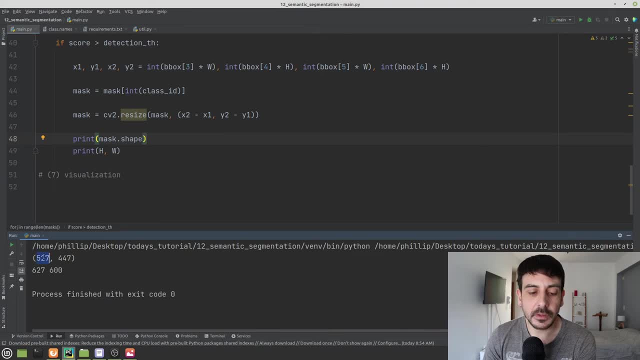 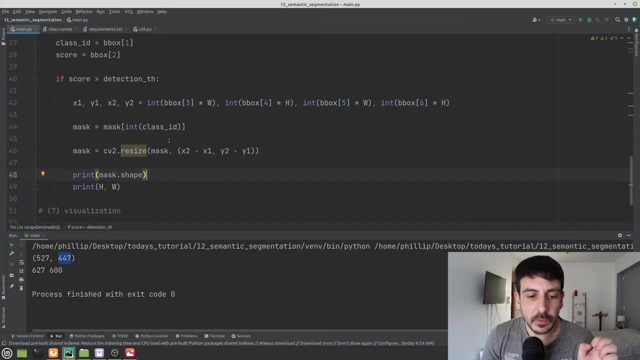 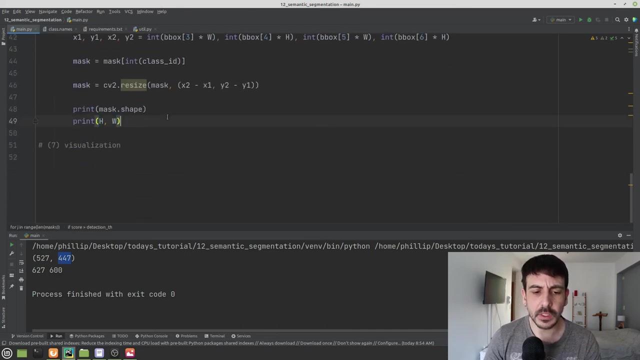 Right, It was 15 times 15, but now is 527 times 447.. So this is the size of our mask, And what we have to do next is to use the empty image I have defined a few minutes ago, And the way we are going to use this image is by doing something like this: 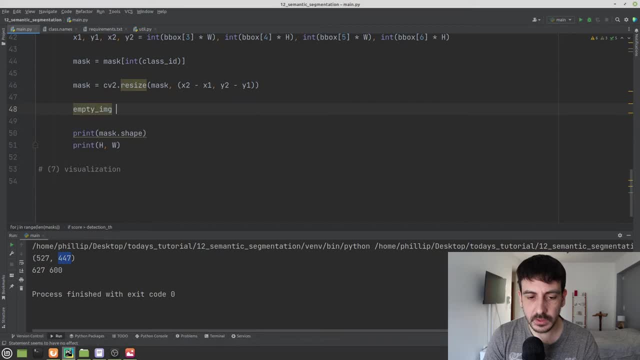 I am going to assigned empty image. This is going to be Y1, Y2.. X1, X2 and something like this, equal to our mask. Now I am going to use this image in order to put the in order to copy my mask inside. 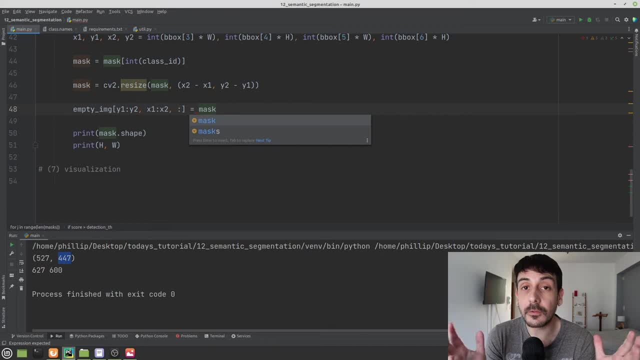 this image. And why am I going to do that? Because I need the information of our mask. I need it in something that's the same size of our original image because I am going to do some, uh, some things in the visualization. 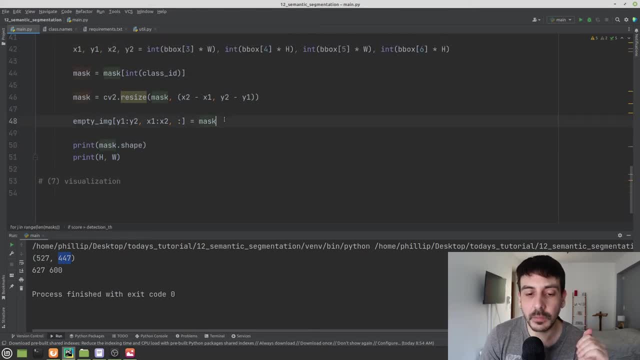 Part of this process and this is going to make perfect sense. So I am going to do something like this, but I'm also going to do something like this: I'm going to assign each one of our channels individually. So for C in range three, this is the way I'm going to do it. 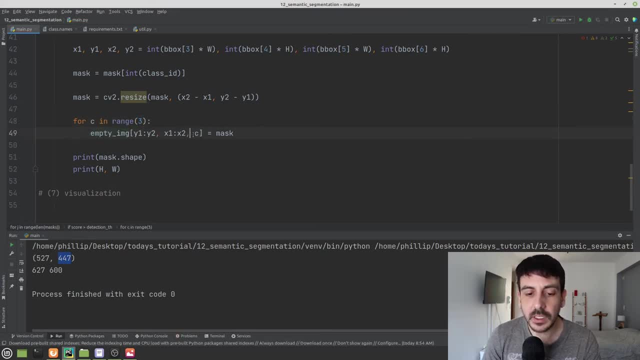 So I'm going to copy or mask in each one of our three channels. So this is a VGR image. We have three channels and this is a grayscale image. We have only one channel. So this is what I am going to do and this should be enough. 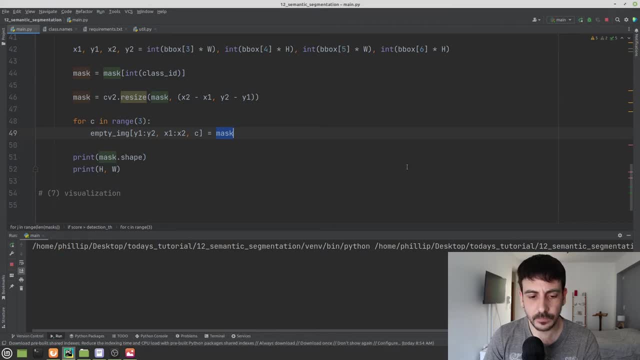 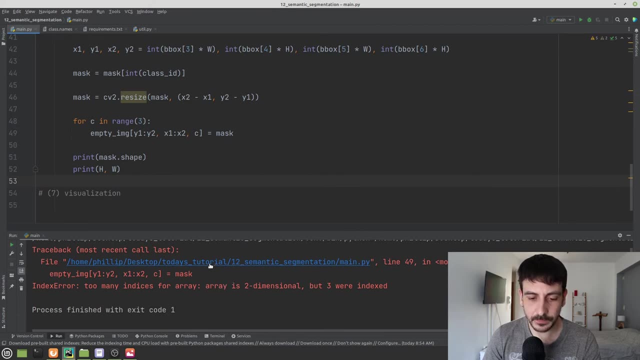 So let's see if everything runs smoothly. Uh, no, everything does not run smoothly. Let's see why. uh, too many indices for Array. Array is two dimensional, but three were indexed Right, So let's define a new index, which is going to be the next. 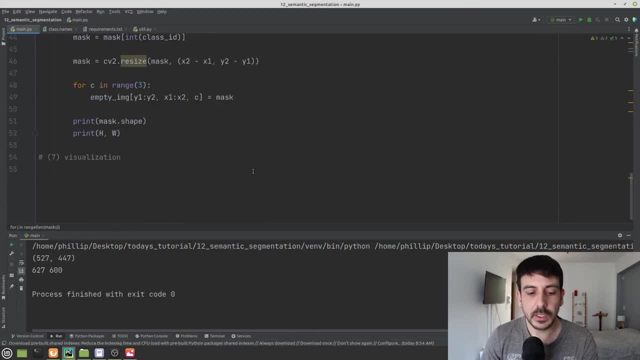 Number of channels, And now everything is going to be okay. Everything is okay, Okay. So we have defined an empty image. We have copied the information of our mask into this empty image. I am very curious to see how this looks like. 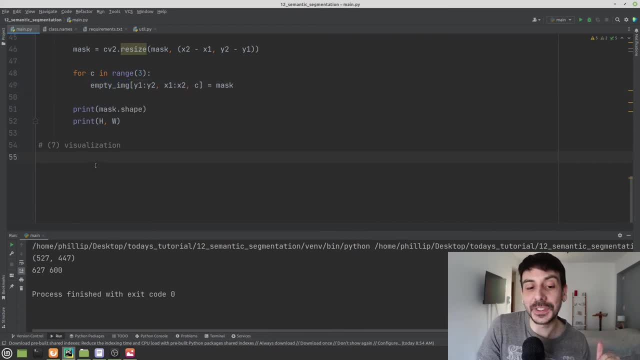 Let's run, Let's move to the visualization part of this process And now let's see how everything looks like. We haven't completed our process. We still have some things to do and we are going to do a little more uh things in this. 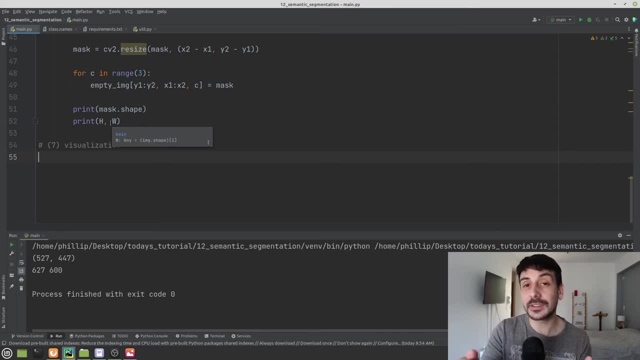 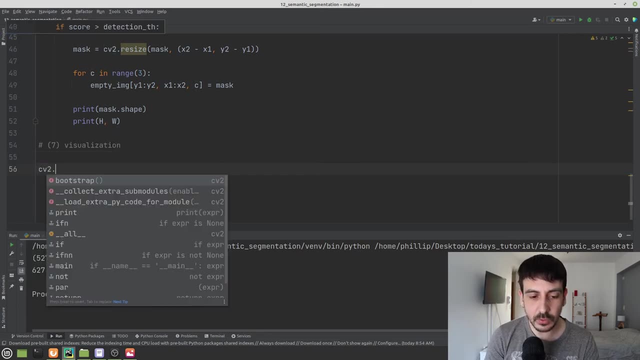 part with the drawing. but let's move forward to the next process, to the next step, And we can always move back to the previous step in a few minutes. So I am going to call CB2 in show and I'm going to visualize the mask. 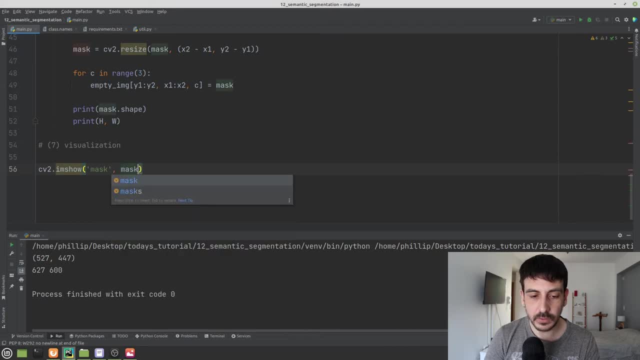 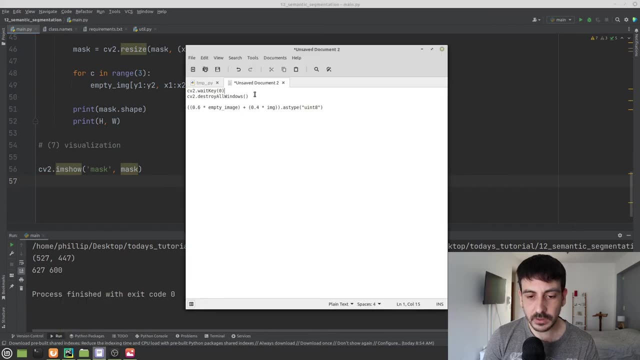 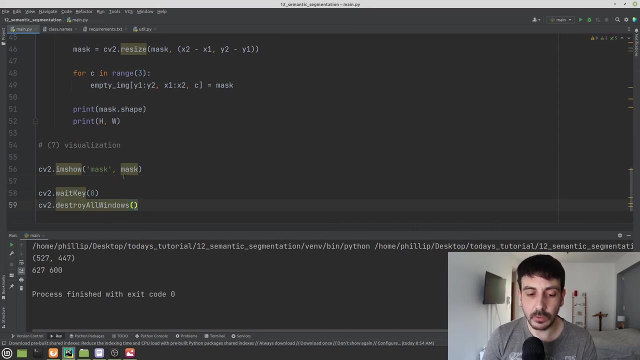 So I'm going to call this mask and I am going to input my mask, Okay, And then I am going to call these two magic lines which are going to make Um, okay, They are going to make everything to hold there until they press any key. 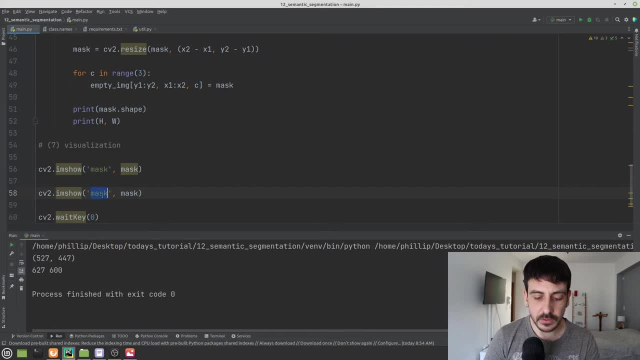 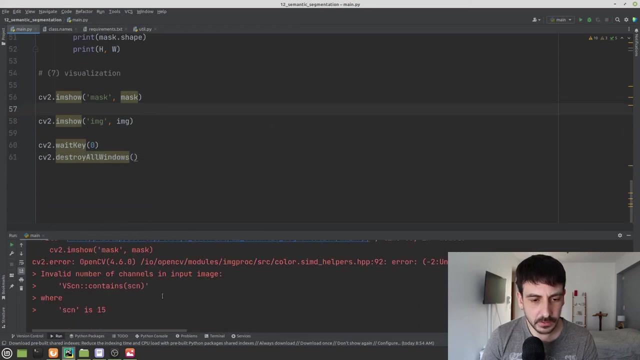 And then I'm also going to visualize the original image, and this is going to be called the image image. Okay, Okay, Let's see what happens with these two visualizations. And then I'm going to plot something else. Okay, Let's see what happened. 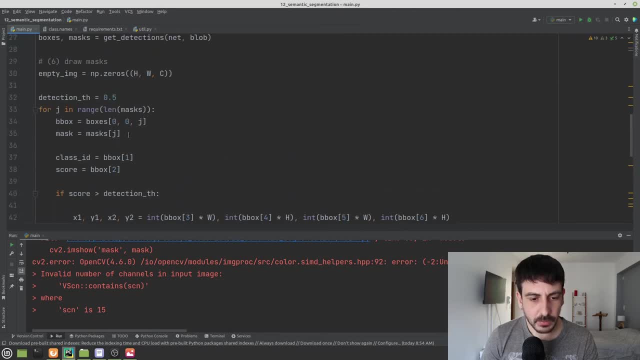 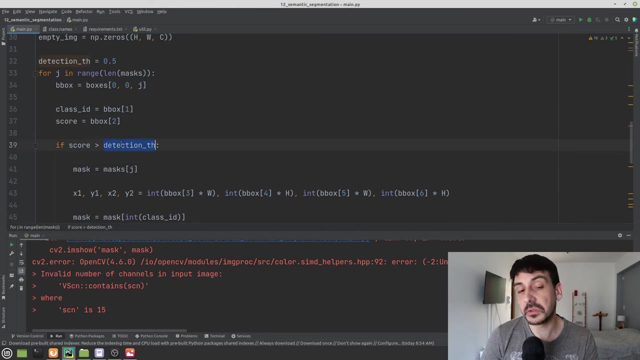 Um, I think I know what. what happened. I think it's going to be a better idea if I take the mask definition here, right, Because we don't really need to define it before. we are going to define it only if the score is greater than detection threshold. it's going to be exactly the same. 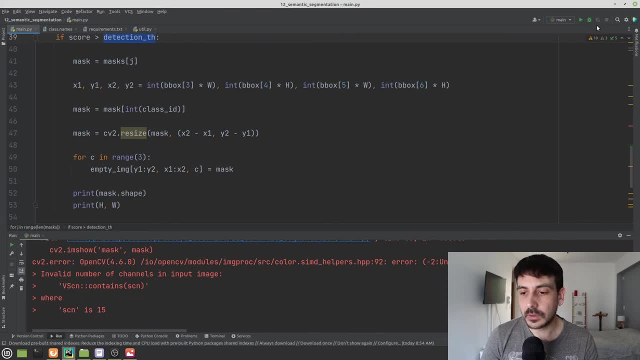 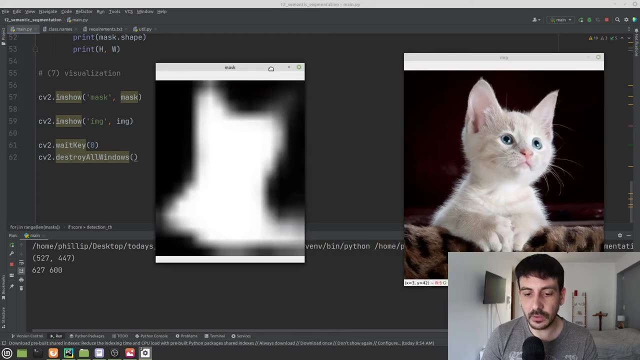 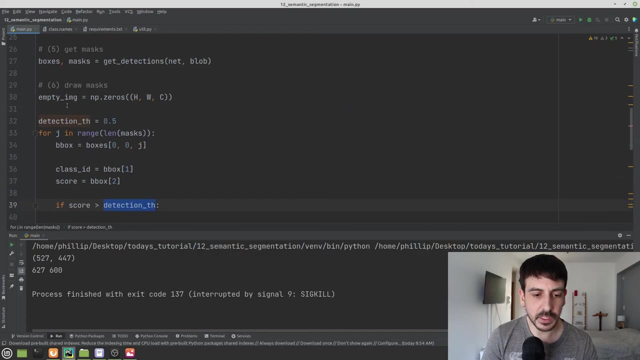 Um, it's going to be much better to do it like this, So let's run it again. Okay, This is our image and this is our mask. Now everything seems to be working fine. I made a mistake instead of um plotting the mask. 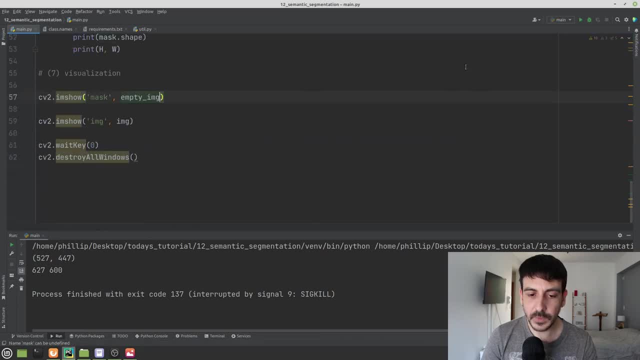 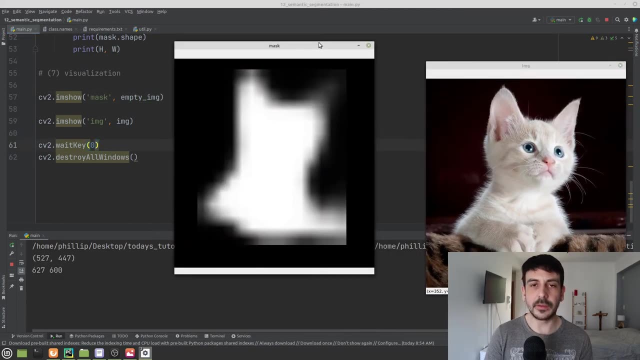 I need to plot the empty image. Sorry, Let's see now what happens. Okay, And now? if I take a look at this images, I see everything is starting to look the way we want it to look. okay, Everything it's like becoming a little more clear. 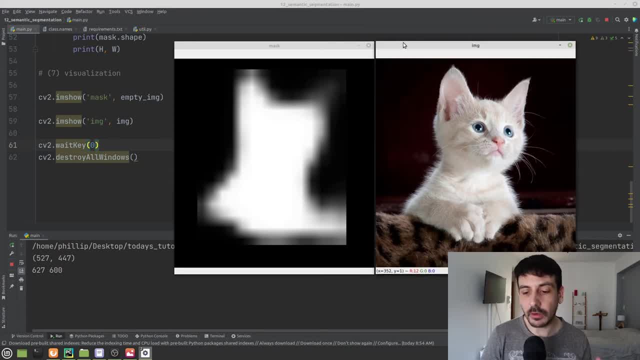 Um, I am going to do a few more things, but you can see that we are almost almost there. Now we have our original image And we have our mask, and the mask pretty much looks like the way we will expect, but we 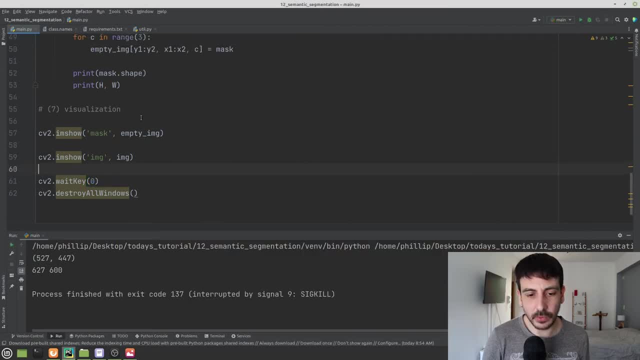 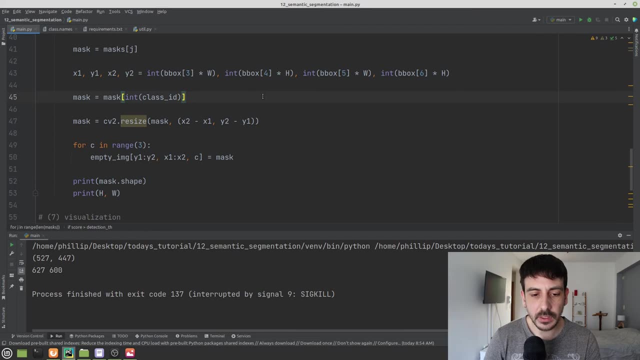 are going to make it even better. So I am going to get back to our code and let me show you what we are going to do. We are going to do something that's- uh, involves the function threshold. So after we do, or resizing, I am going to do something like this: mask is now equal to 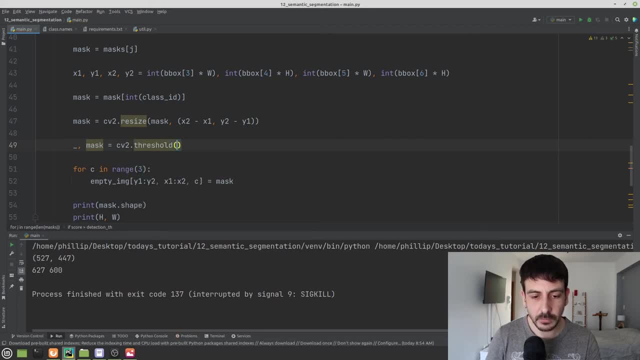 uh, CB two threshold. Oh, And I am going to input the uh image or or mask, And I am going to input the um, this number, 0.5, then one, and then this is going to be. 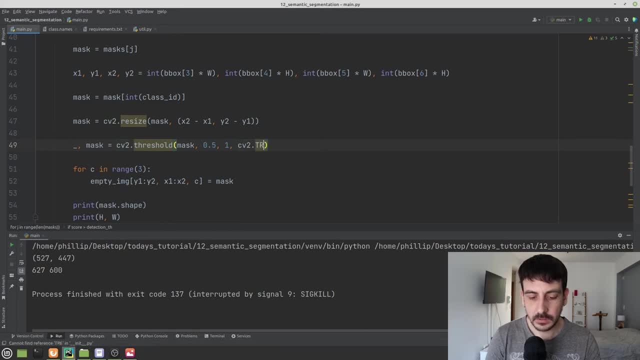 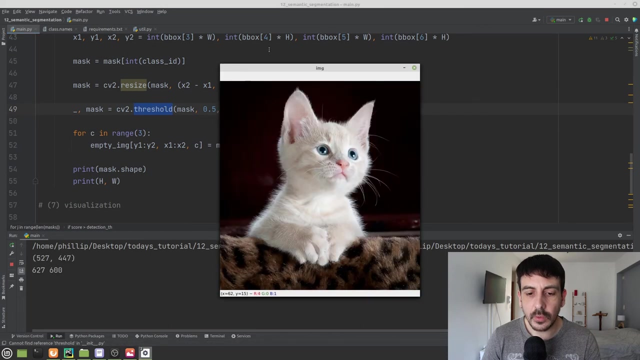 CB two, dot tres, the tres binary. Okay, Uh, so this is it. Let me press play. What we are going to do, Call in threshold Is that? Uh, we are going to take absolutely all the pixels in our image and we are going to make 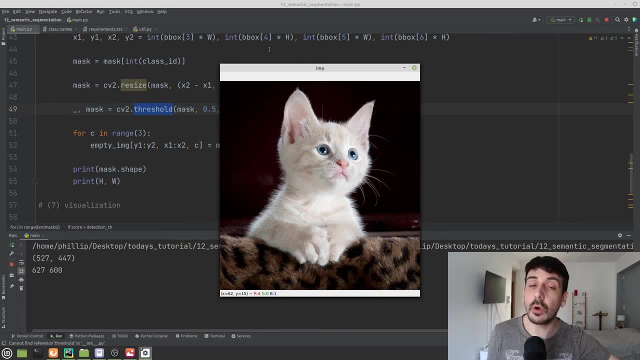 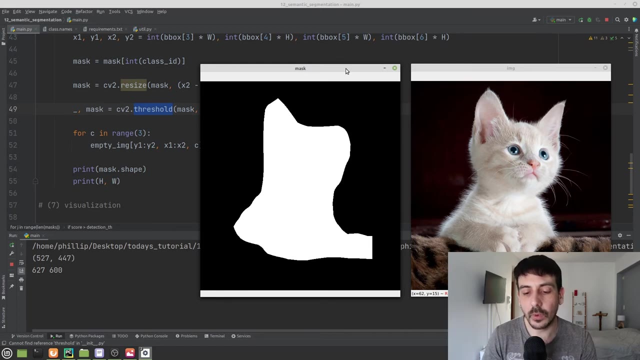 absolutely every, every single pixel, to the value of zero or to the value of one. We are going to make absolutely everything to be either black or white. So let's see now how our mask looks like, And you can see that now we have something that's more the type of mask we were expecting. 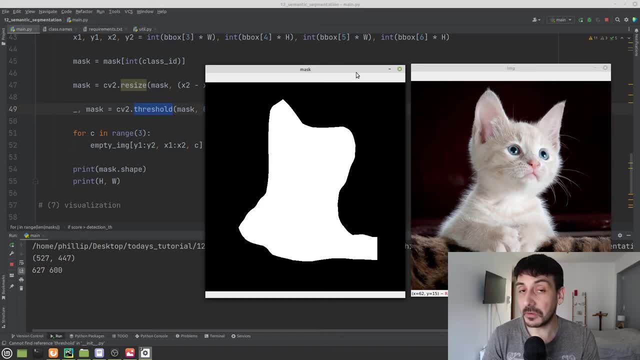 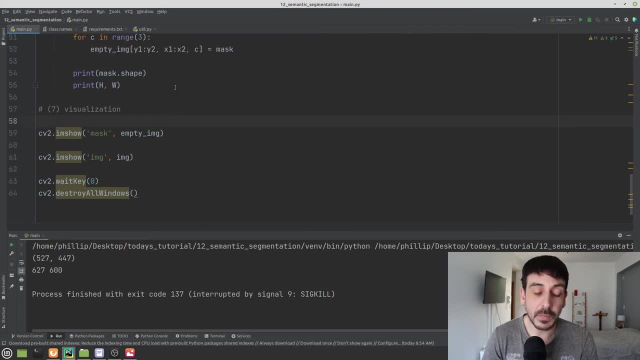 to get right. So everything seems pretty fine if you ask me. But what we are going to do in order to have like a better visualization, is to define another, uh, another image, which is going to be called overlay, and overlay It's going to be called, it's going to be defined as this value. 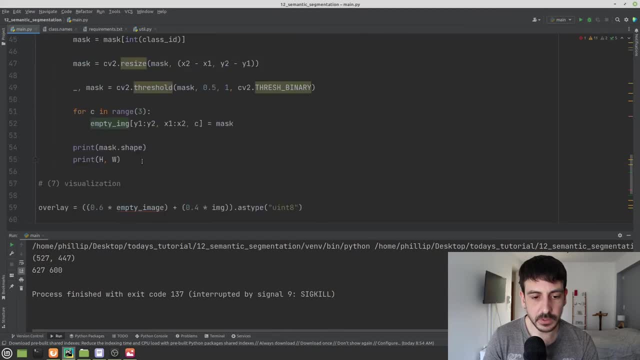 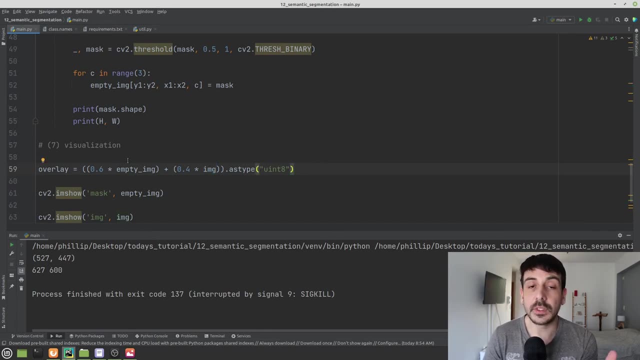 Okay, So this is my empty image and this is my image. This is pretty much the only thing we are doing with this sentence, with this definition, with this new overlay. Okay, So we are going to do overlay, or two images. We are just going to plot one of them on top of the other. 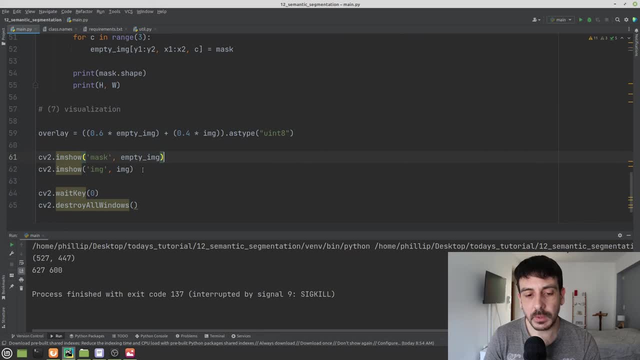 So this is going to be a very good uh tool, that these are going to be a very good way in order to see how they look like together. One on top of the other. this is going to be overlay, and this is going to be overlay. 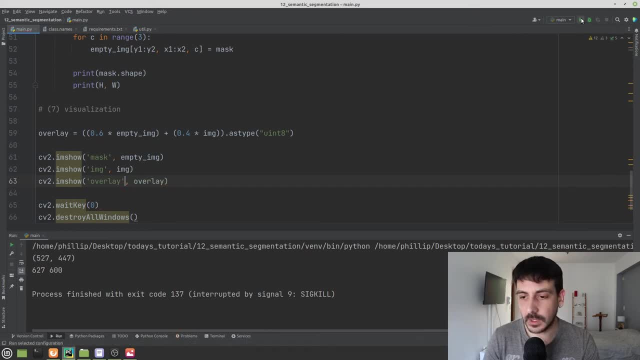 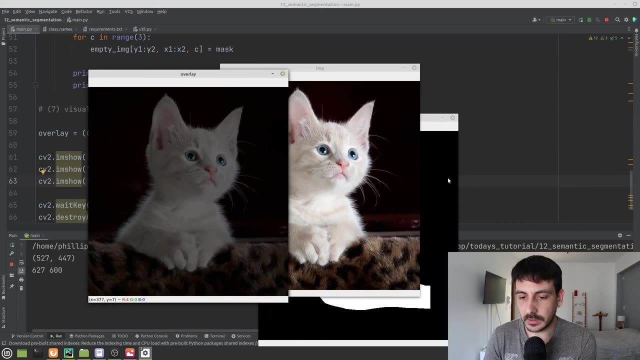 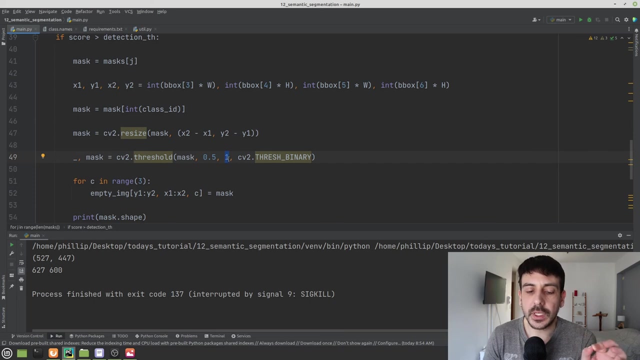 too. Okay, Let's see now how everything looks like: Uh, something. Okay, This is not right, And I know what. what is it? Uh, there are two different ways in which we can do this. We can either, uh, take everything to the value of one, or we can take everything to. 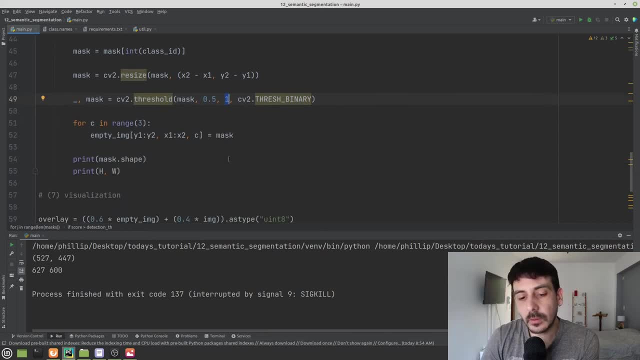 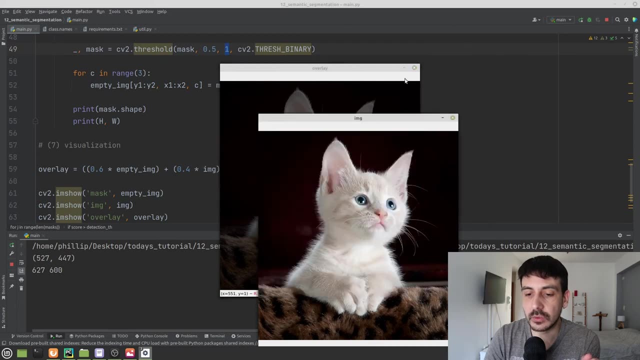 the value of 255,. uh, either way, we are going to be okay If we want to visualize only the mask, only that individual image. if we want to visualize this uh image, it's going to be exactly the same. 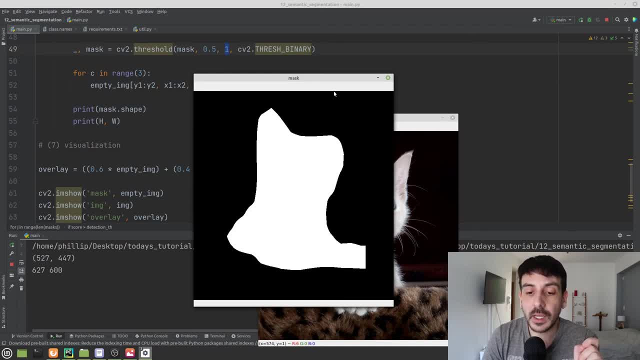 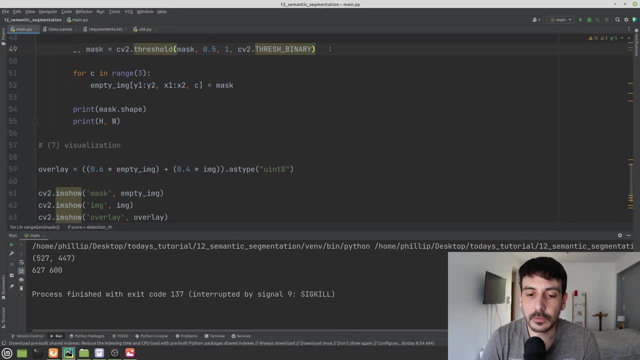 If we take it to one or two, 255.. But as we want to make this overlay, it's going to be much, much better if we take everything to the value of 255.. So, uh, maybe the best way to do it is something like this: mask is equal to mask times 255. 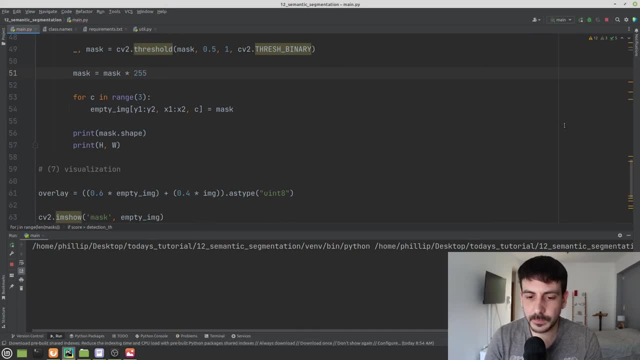 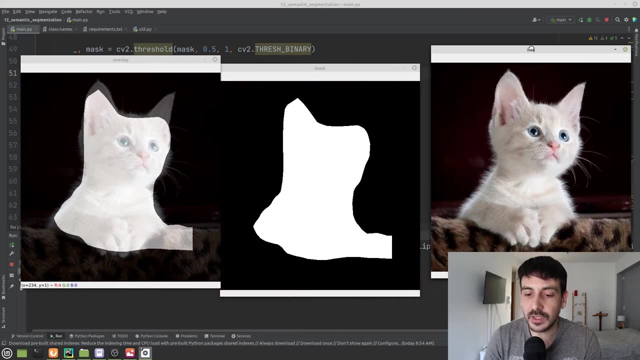 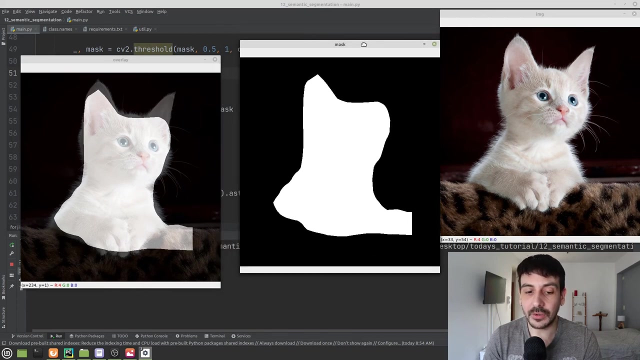 Let's see if this works. And this works pretty well, So you can see that this is our original image. This is our original image. Then this is the mask we got from this semantic segmentation algorithm And this is the overlay of this mask, with this image. 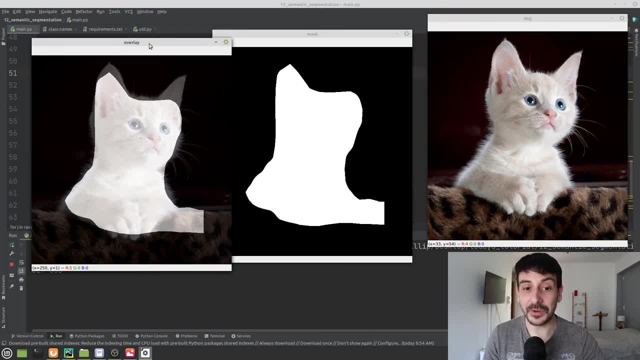 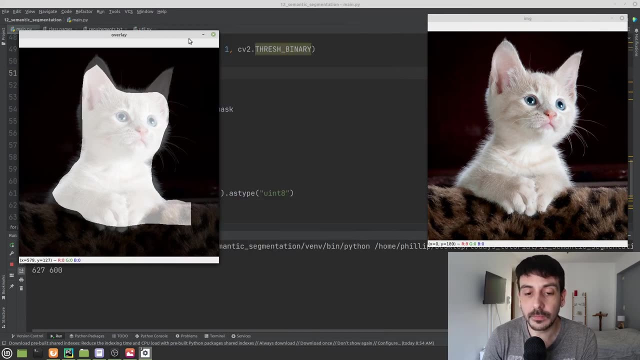 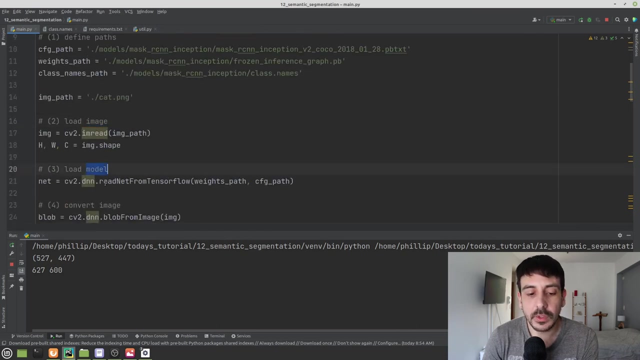 And you can see they match perfectly. We have detected or object or cat perfectly, So this means that we are pretty much there. Actually, we have really much completed this tutorial and you notice how simple this was. Okay. So what we needed to do is to define our model, to define our image, to load our image then. 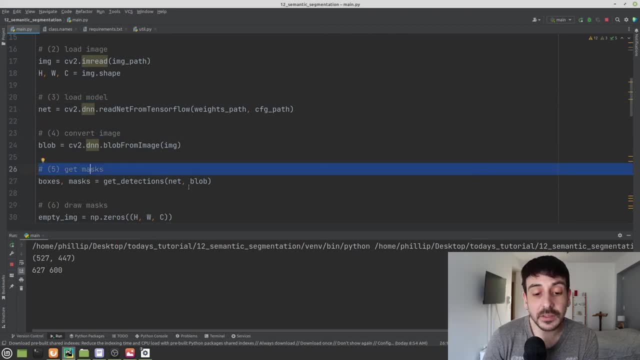 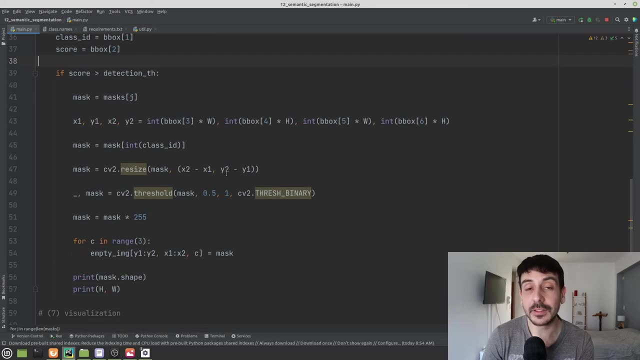 loading our model, then converting our image, Then we just got the masks calling this function And then we draw the masks. that, if I have to be honest, yes, it's true that this was a little more complicated than everything else, but anyway, it wasn't really that complicated. 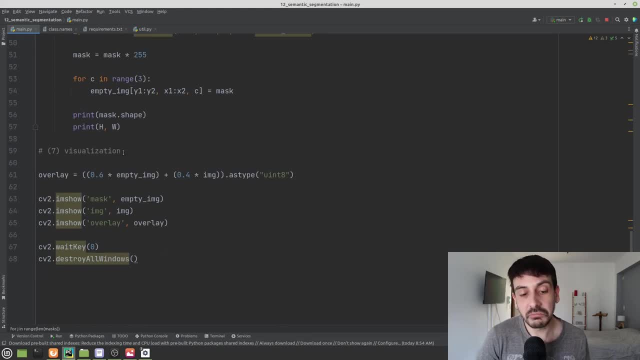 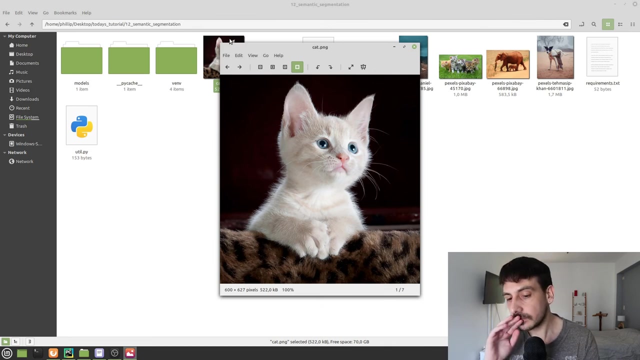 And then, when we wanted to visualize our images, we only had to call this. So this is going to be pretty much it, but I am going to show you something else, because in this image we have only one object, We have only one cat. 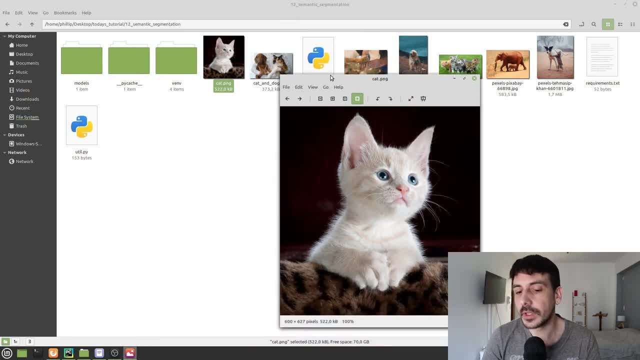 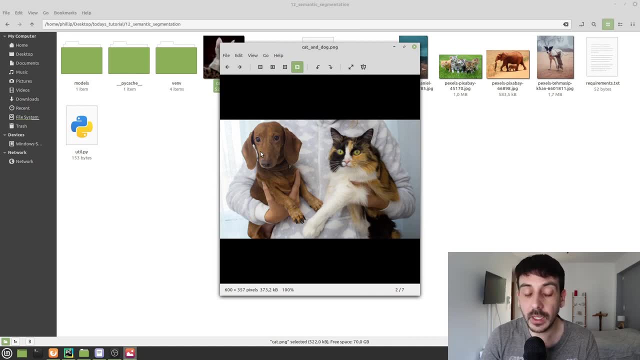 What happens if we want to visualize more than one object? What happens if we want to visualize, for example, the masks for these two objects? Now, here we have a dog and we have a cat. What happens? How can we achieve to have a cat? 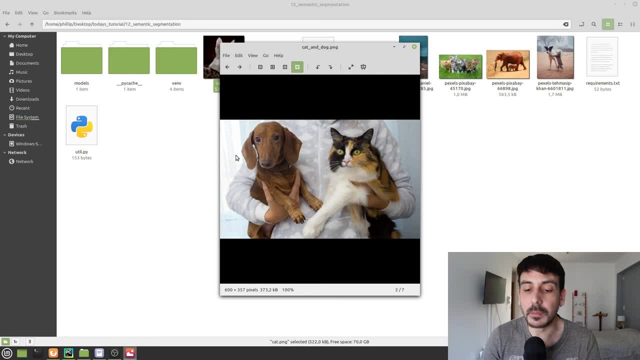 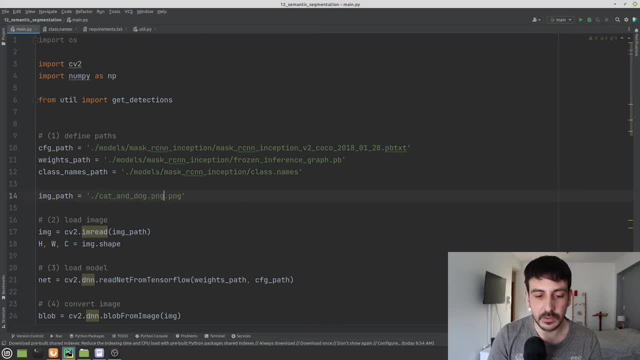 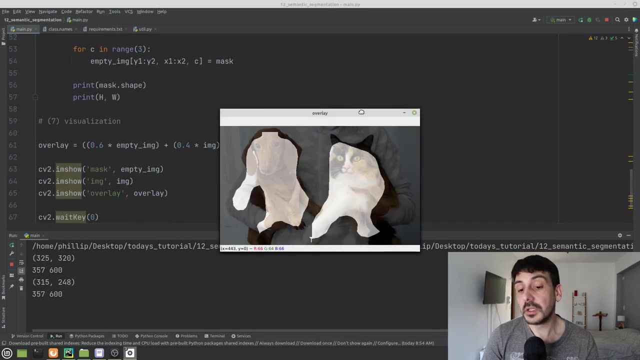 Okay, We have a visualization of these two masks, So let me show you what happens if I just replace our image by this other one and I press play. I wait a couple of minutes and if I press play, you can see that it works perfectly. 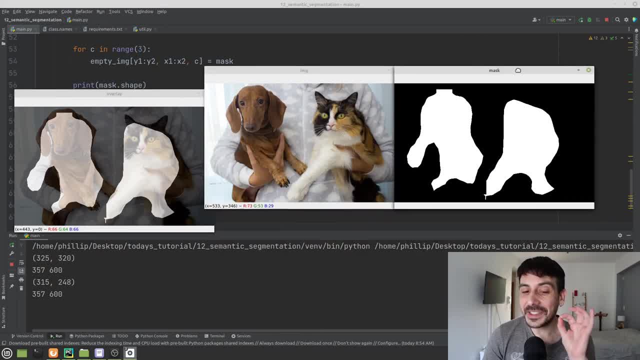 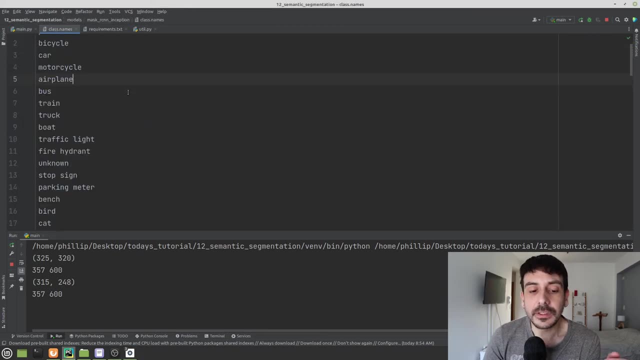 It works very good too, But the only detail in this visualization is that we are getting two masks, and both of them for the same, with the same color. Ideally, if we are detecting different objects, if we are detecting 90 different objects. 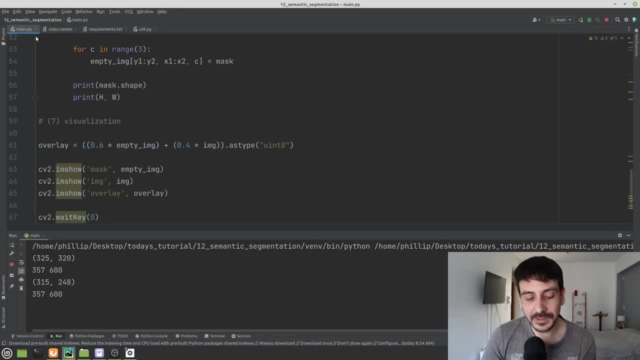 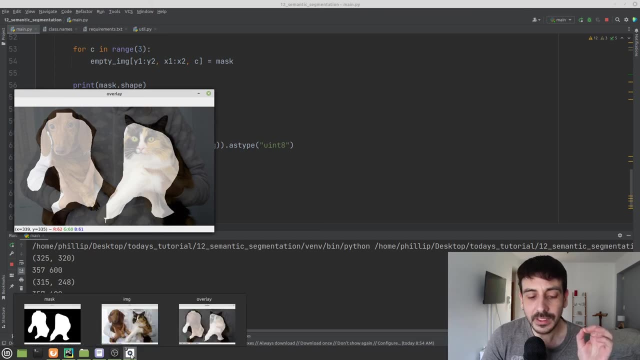 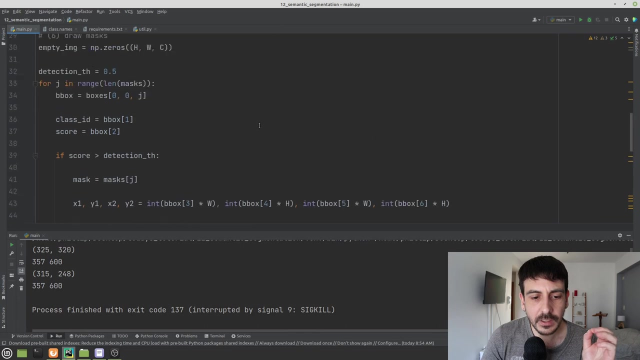 as we are doing here, we will want, ideally, to have different colors for all the different objects we affect. So let's just do that detail, Let's just fix that very, very small detail, And what I am going to do is define a new variable which is called. 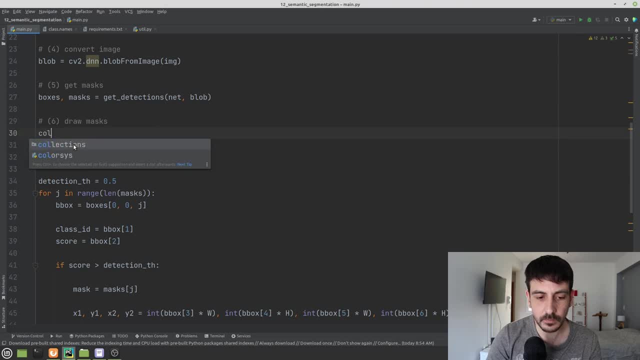 Colors, and colors is going to be a list of random colors, completely random colors. So each one of our colors is going to be something like this: Okay, For J in or class names, We can say: for J in ranch 90, because that's how many. 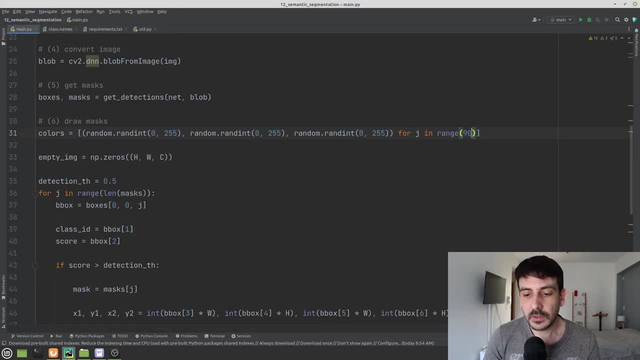 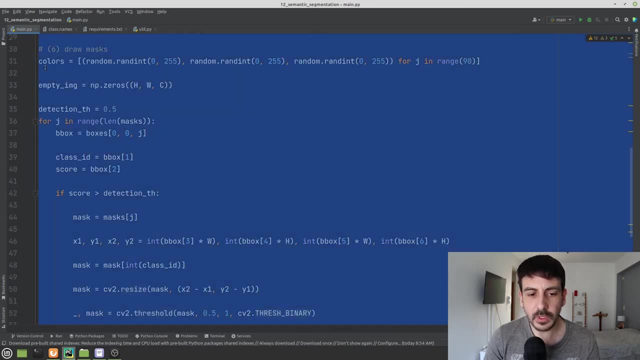 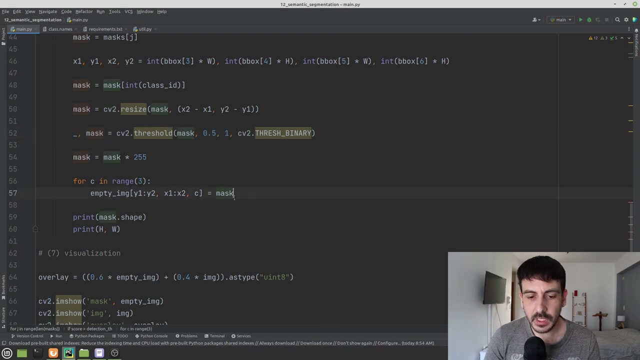 Okay, How many classes we have right, So we can say something like that and it's going to work, Yeah, So let's just define this new variable And then what I am going to do is, when we are copying or image, what I am going to do. 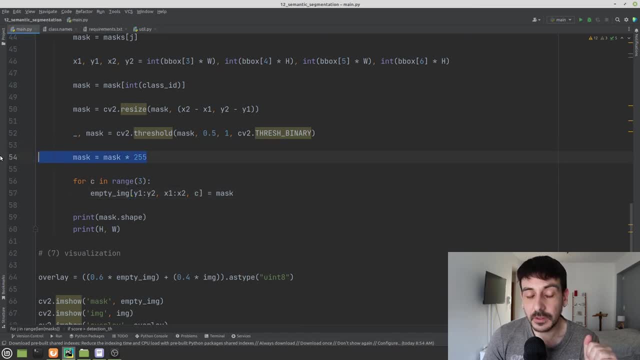 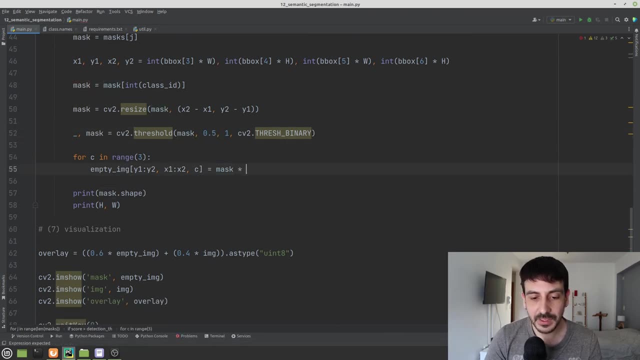 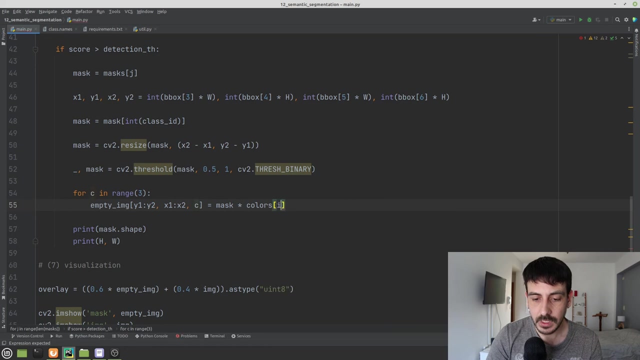 is, instead of multiplying everything by 255, which is the way we got white- I am going to multiply everything Time By the color names, The uh callers, E and glass ID And then see right. Yes, because for each one of these channels I want to copy the information for mask, but 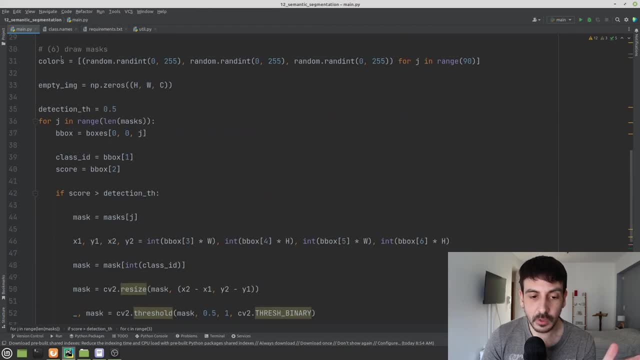 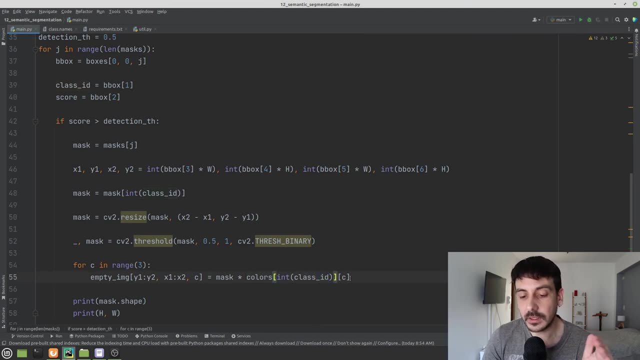 in this color, which is going to be Callers, of the object defined by the uh in this position, which is the, the classic as we have detected, and then the um, the channel c. so this is going to be enough in order to have 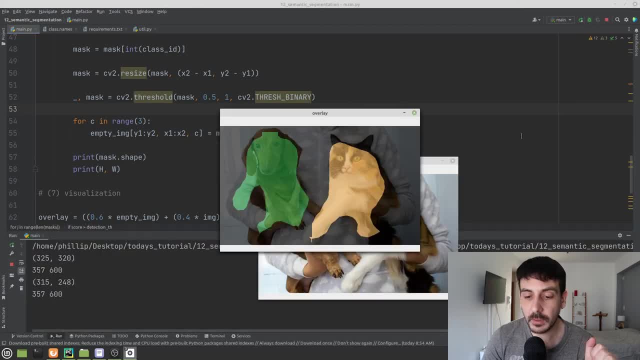 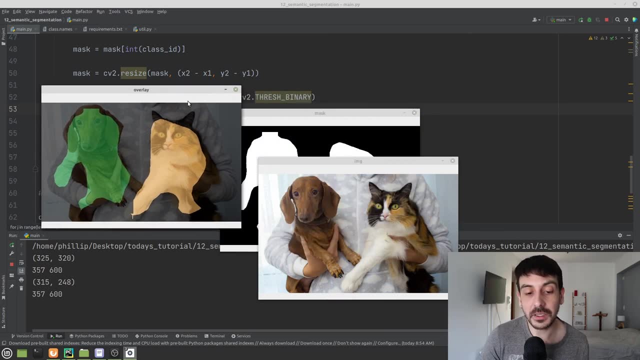 math or masks for from different colors. and let's see what happens if i press play again. and now you can see we are still detecting all of our objects and we are getting exactly the same masks, but now in a different color for each one of our objects. and every time i execute this 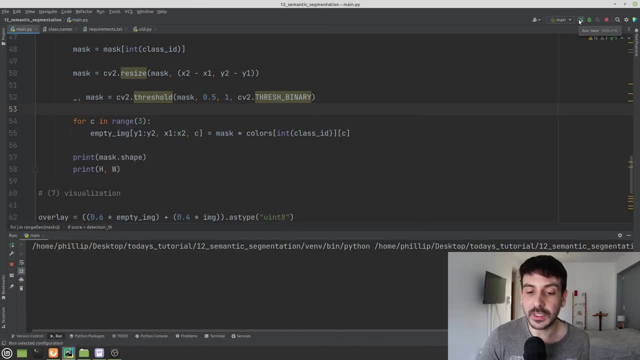 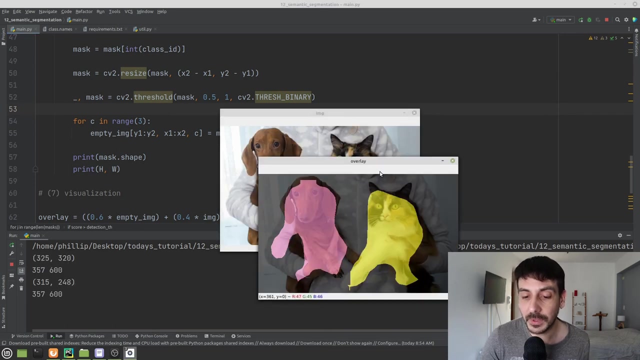 function, we are going to have a different visualization. for example, if i execute again, we are getting the: these two colors are very similar. this is only a coincidence. let me show you again: as these are random colors, we could perfectly, it will perfectly happen that the colors are very similar, but now it's not the case. so in this case, for example, one of our 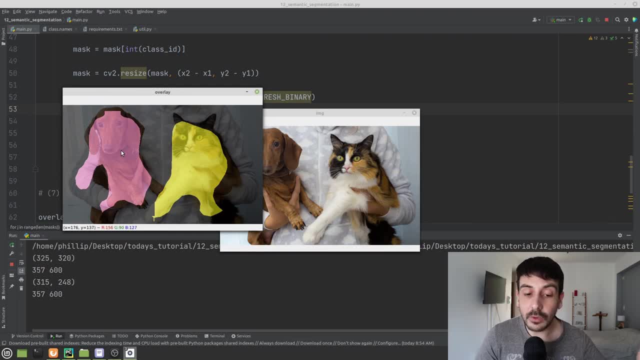 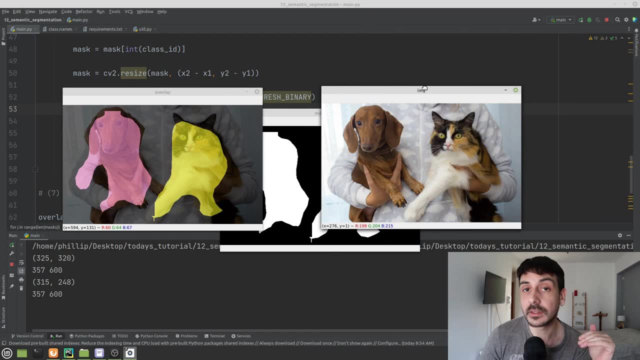 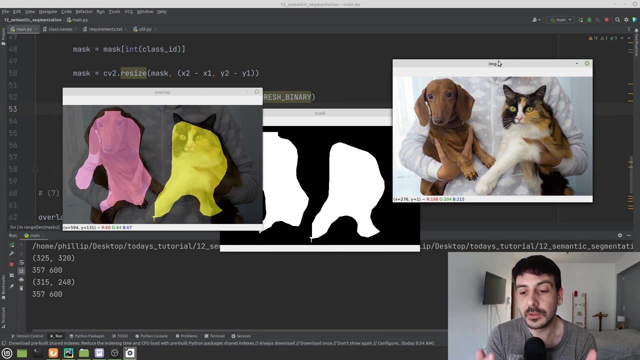 objects is yellow, the other one is red, pink or something like that, and if i continue executing this function is going to happen exactly the same thing: every new object that we detect is going to be detected with a different color. it's going to be plot with a different color. so this is going to be all for this tutorial. this is how you can. 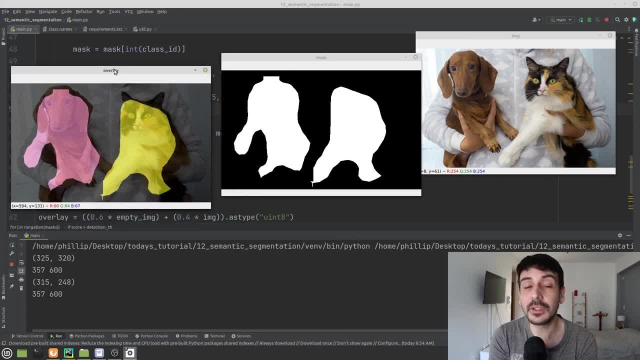 implement a semantic segmentation algorithm using python, tensorflow and opencv, and this is a very easy, very fast and very straightforward way to implement a semantic segmentation algorithm. i will say it's the easiest way to do it, so this is going to be for this video. my name is felipe, i'm a computer vision developer and in